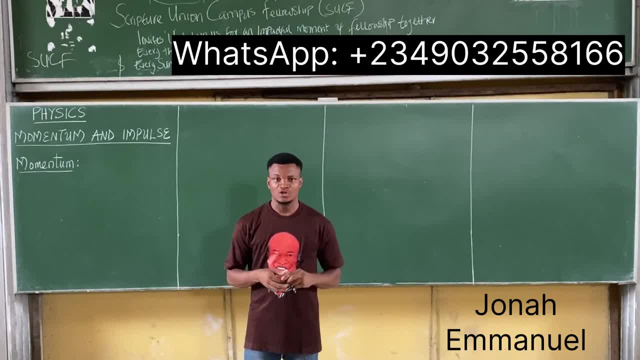 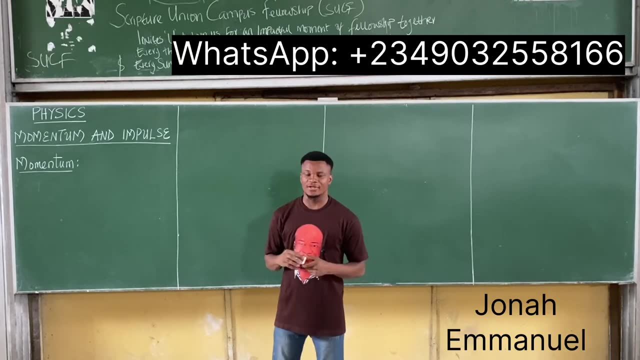 mass of the body and its velocity. So by definition, we can say that Momentum is simply the product of the mass of a moving body and the velocity with which the body moves. Something to note is that Momentum is represented with a small p, So in physics we represent Momentum. 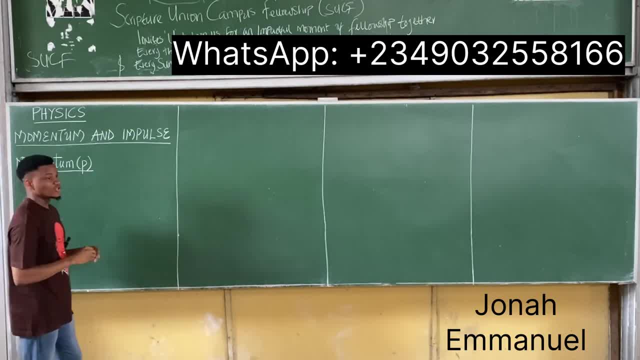 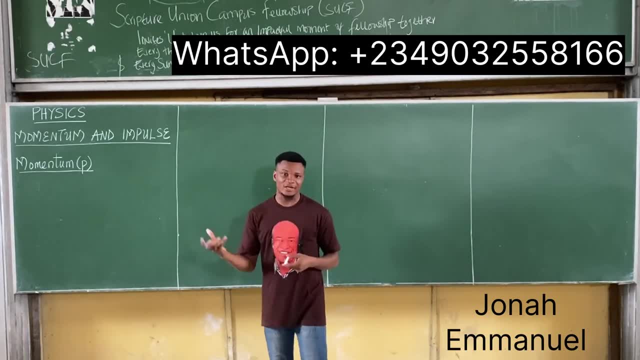 using a small letter p. So small letter p is for Momentum. The capital P obviously is for Pressure. So Pressure is capital P and Momentum is small letter p. And you might want to ask why is that? Momentum is not m? The idea is that m. 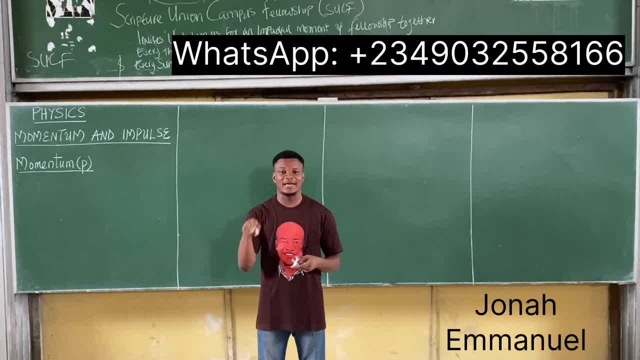 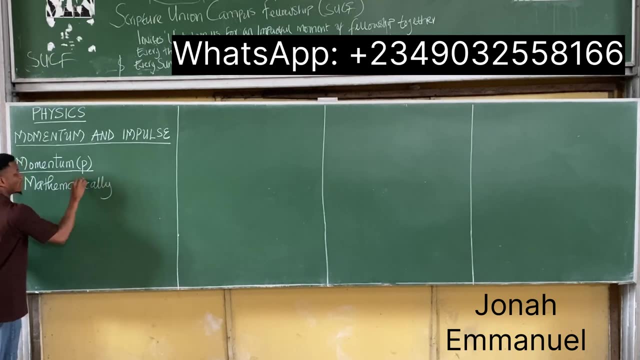 already represents mass. So whenever we see m, small letter m, it's usually mass. So, having said that, we are using small p to represent Momentum in physics. So, mathematically, mathematically, mathematically, let's say we have a body of mass, m, moving with a velocity. Let's say the velocity is: 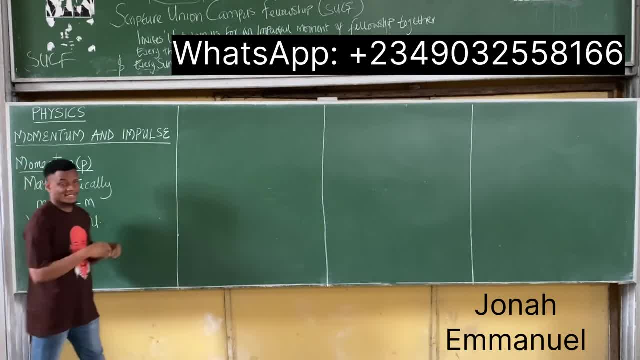 about. we can call it u or v. Let's use u, or we can say v, if you want to. Well, it's saying that the Momentum p of the body is equal to mass times velocity. Hence, Momentum is equal to mass times velocity. So we have this All right. So this becomes the formula. 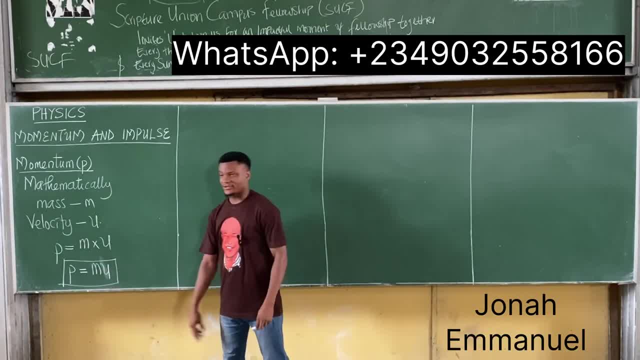 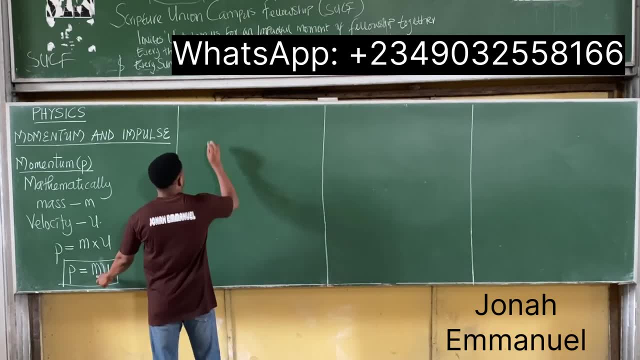 for calculating Momentum. All right, Mass times velocity. Now, if this is the case, let's get the SI for Momentum. Now we just said Momentum is mass. All right, Mass is measured in kilogram and, of course, velocity in meter per second. Hence we can say: the SI unit, the SI unit of Momentum is: 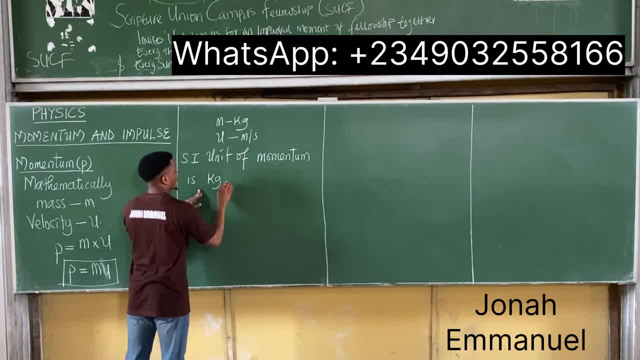 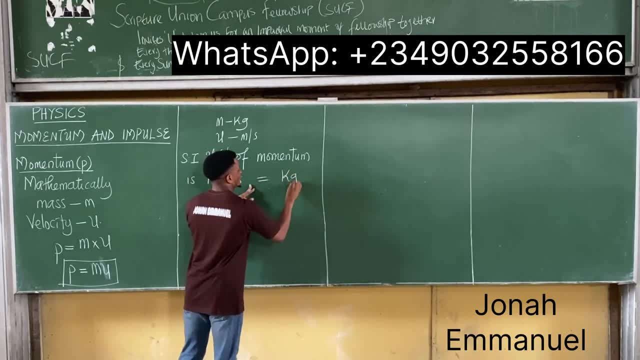 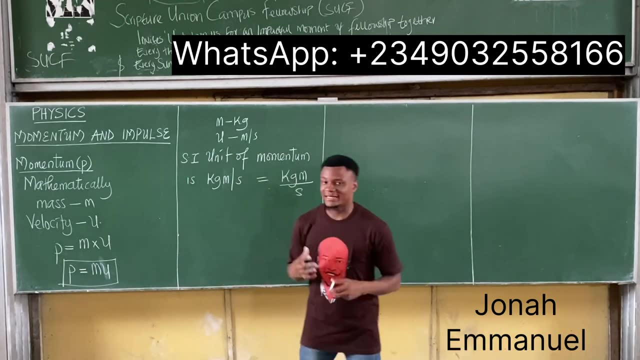 kilogram Me meter. kilogram meter per second. So this is the SI for Momentum. It can still be written as kilogram meters all over second, All right. So this is the SI in its form, Momentum. Now let's take a problem, a sum problem. So solution: let me take a question here. So, 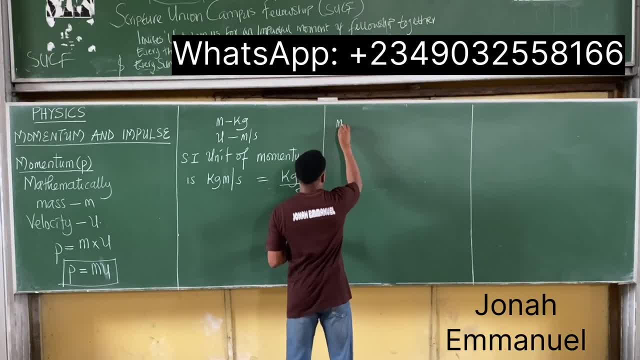 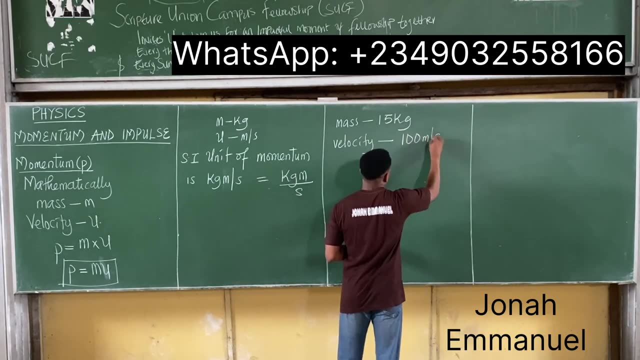 let's say we have a body. let's say we have a body of mass, Let's say 15 kilogram, moves. moving with a velocity of, let's say, 100 meters per second. So I have a body of mass: 15 kilograms. 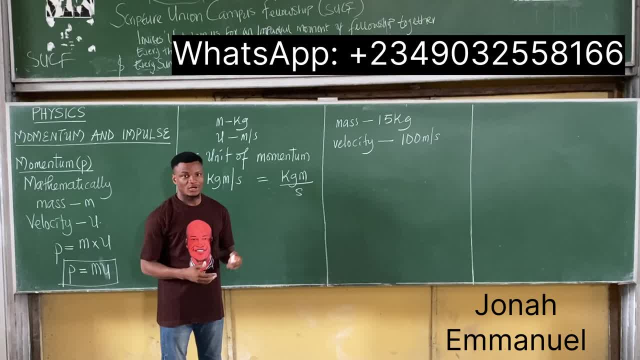 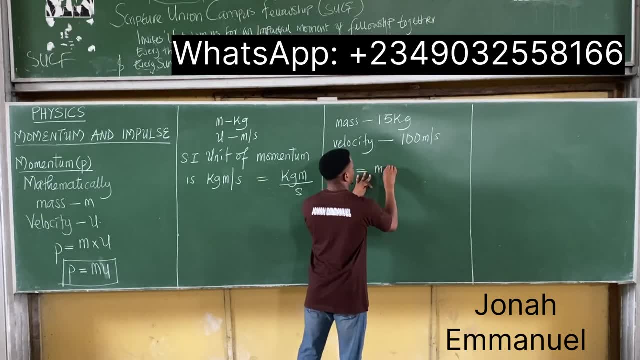 moving with a velocity of 100 meters per second. For this, the momentum P of this body is equal to the product of its mass times. velocity, Hence, that will be equal to mass, is 15 times velocity is 100.. If I multiply this, I have 1,500. 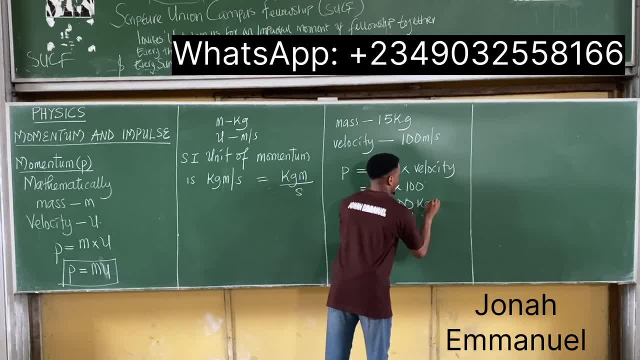 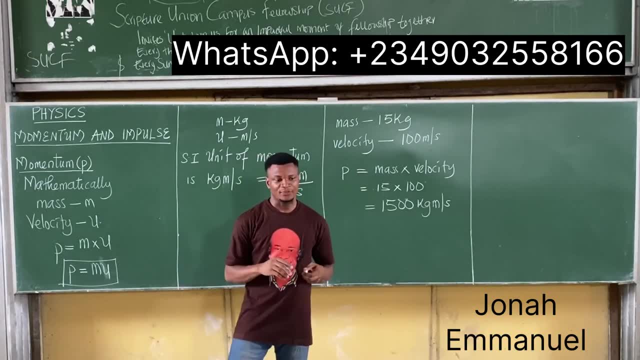 Bring back my unit, which is kilogram meter per second. All right, so this is just a simple concept of momentum, all right, The product of the mass of a moving body and the velocity with which the body, the body, moves. that's it. 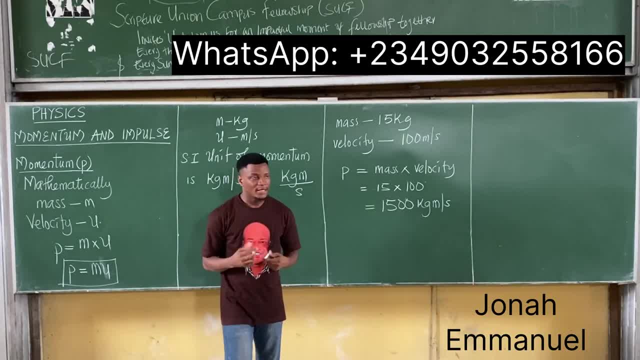 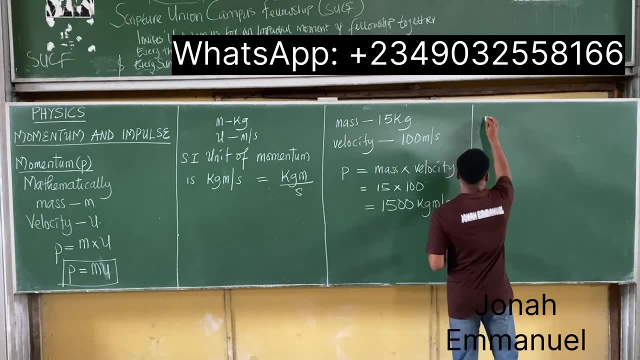 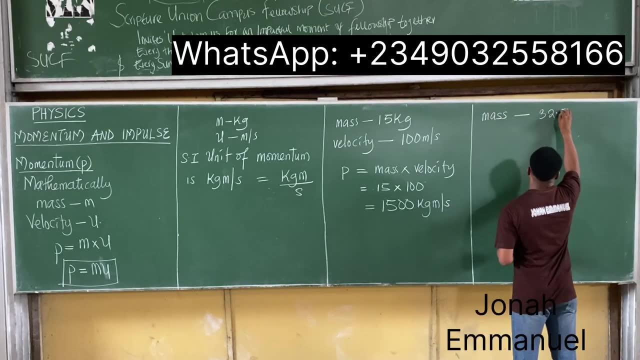 Let's take one more question on momentum and see how we can solve yet another problem on momentum. So let's say we have a body of mass, Let's say we have a body of mass 32.5, okay, Let's say the mass about 32,500 gram, right? 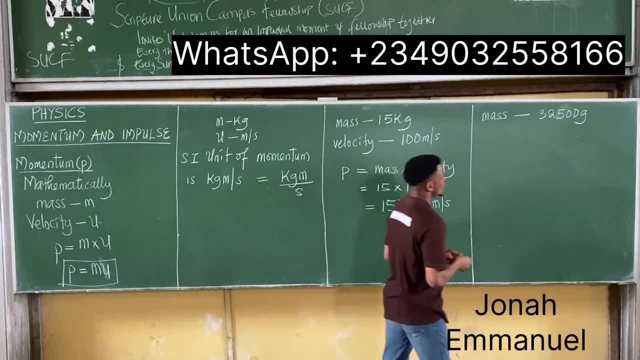 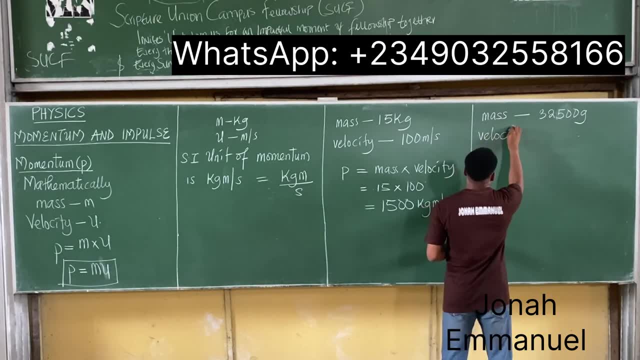 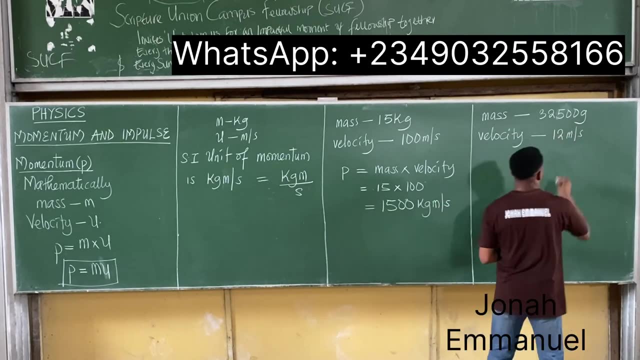 Let's say we have a body of mass 32,500 gram, moving at a speed of a speed or a velocity of, let's say, 12 meter per second. all right, A body of mass 32,500 grams. 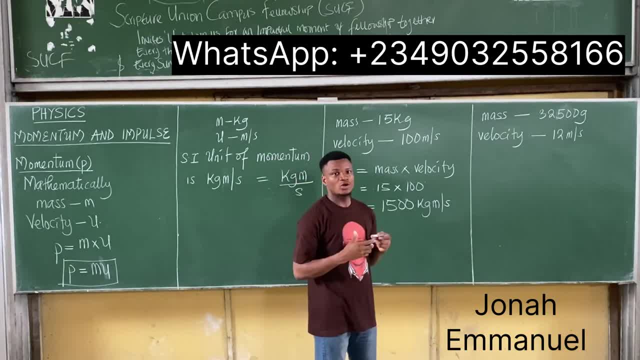 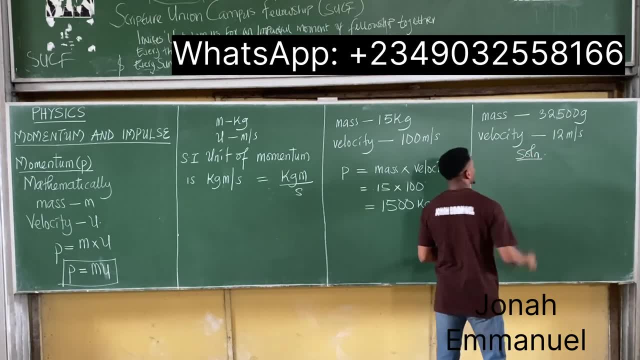 moves with a velocity of 12 meter per second. What will be the momentum For this? it's as simple as this. My solution: first things first. mass m is equal to 32,500 gram. Now, first things first. 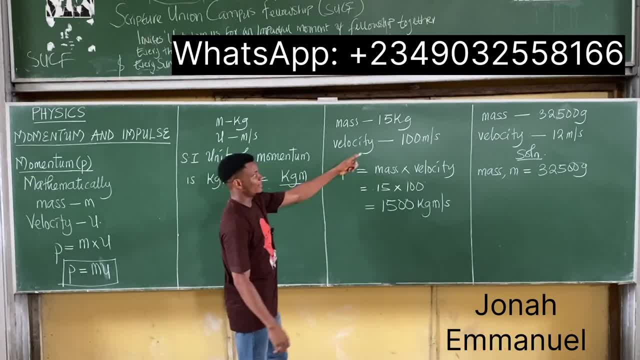 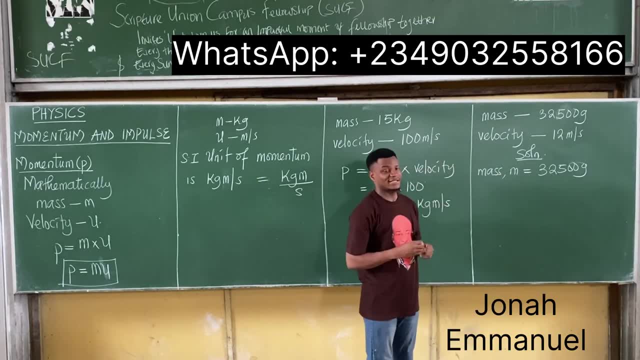 recall that mass is measured in kilograms, not gram. So the question is: if I have my mass in grams, how do I convert to kilograms? It's as easy as dividing by 1,000,. all right, If we divide by 1,000, you have the value in kilograms. 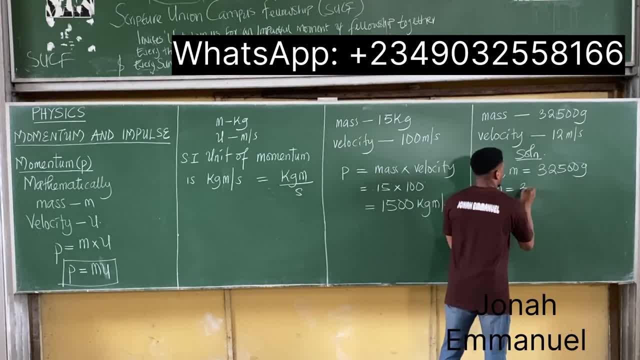 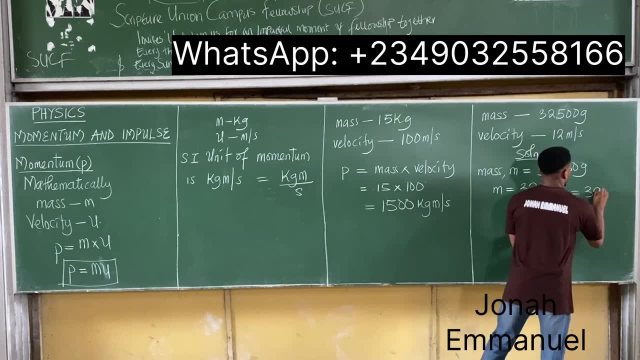 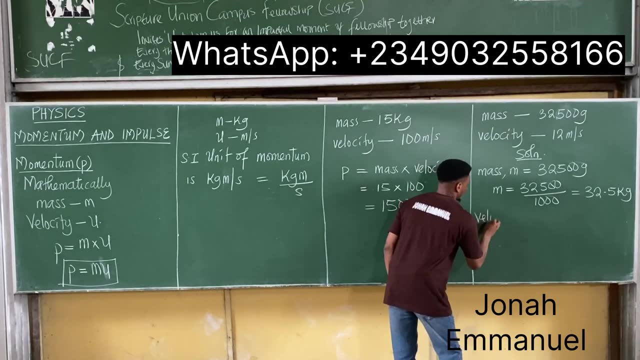 So for this the mass becomes this value: 32,500, divided by 1,000.. That will give you about 32.5 kilograms. So you have this. Also. velocity has already been given as 12 meters per second. 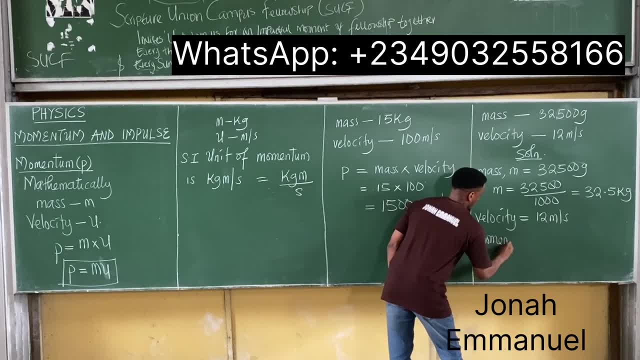 Hence we can say that the momentum, the momentum of this body is equal to. the momentum of this body is equal to. the momentum of this body is equal to 32.5 multiplied by velocity, which is 12.. And that will give you about. 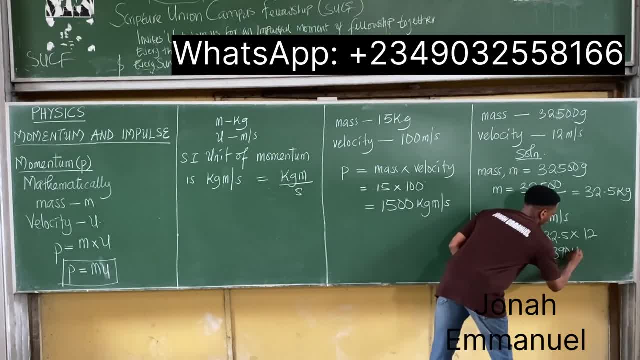 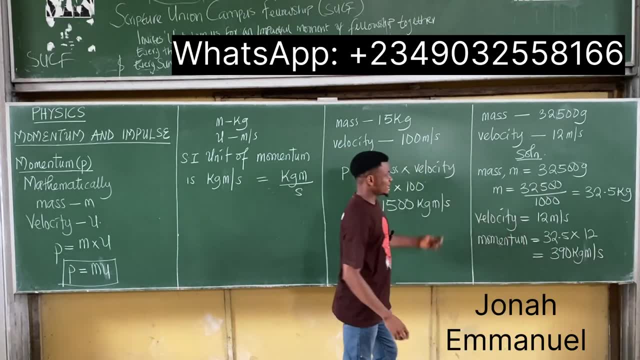 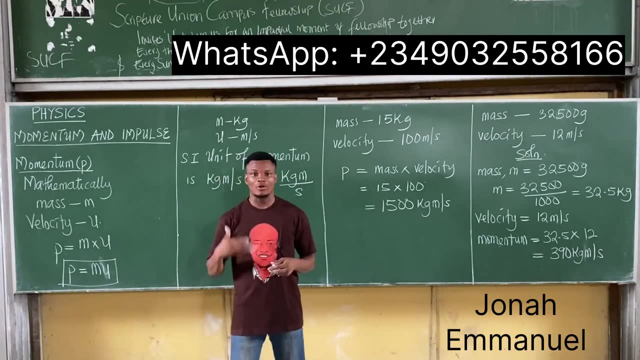 about 390 kilogram per kilogram. meters per second. All right, So this is a simple concept about momentum. We'll look at the concept of conservation of linear momentum much more later, But before then let's consider the second concept, called impulse. 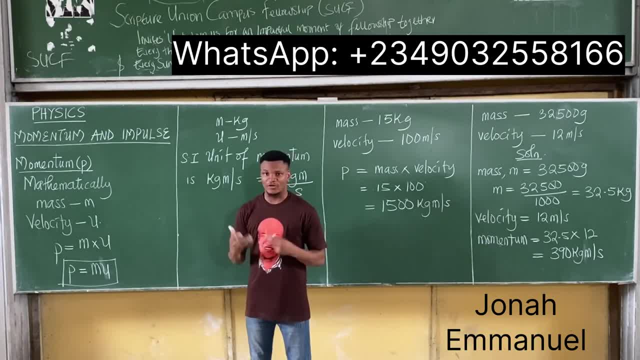 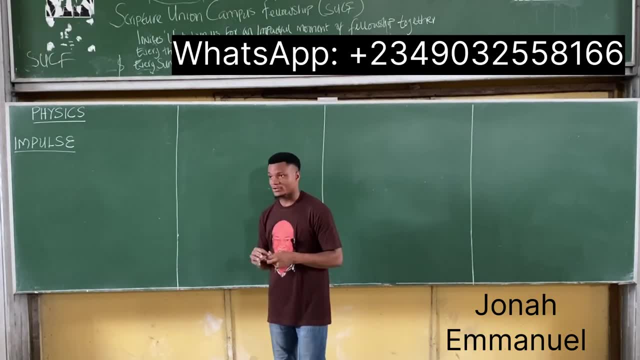 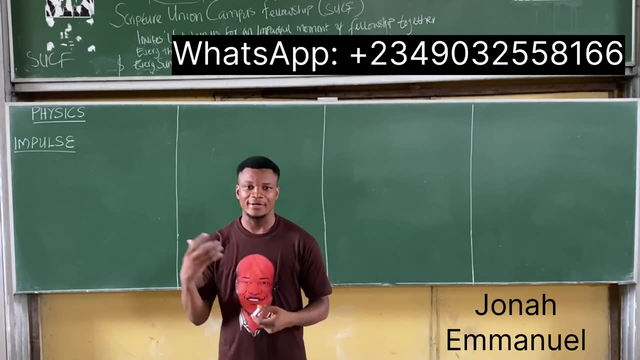 So we look at impulse, look at what it means and then solve some little problems on impulse. All right, so let's look at the next concept: impulse. By definition, impulse is simply the product of the average force acting on the body or a particle. 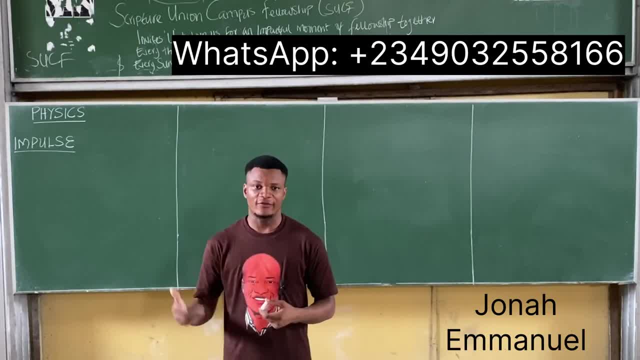 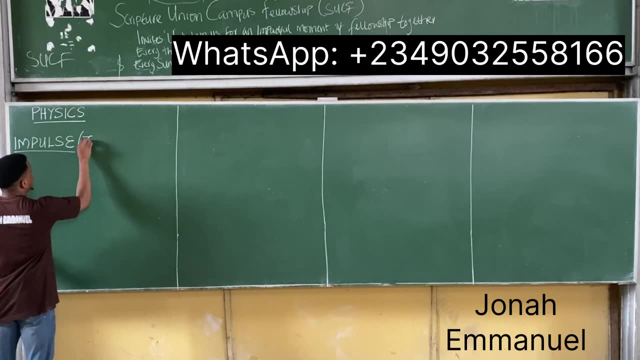 and the time interval within which the force acts. all right, The product of the average force acting on a particle, a body and the time interval within which the force acts. alright. When it comes to impulse, note that impulse is generally represented by using J: alright, J represents impulse. 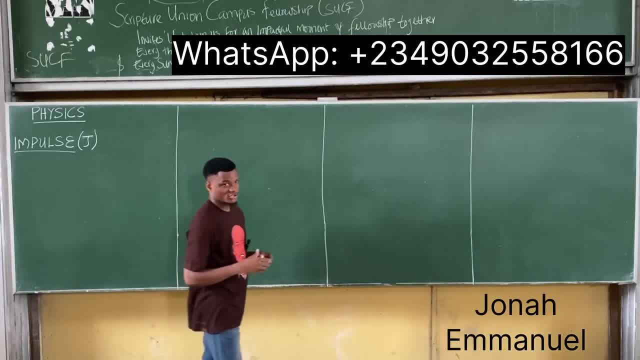 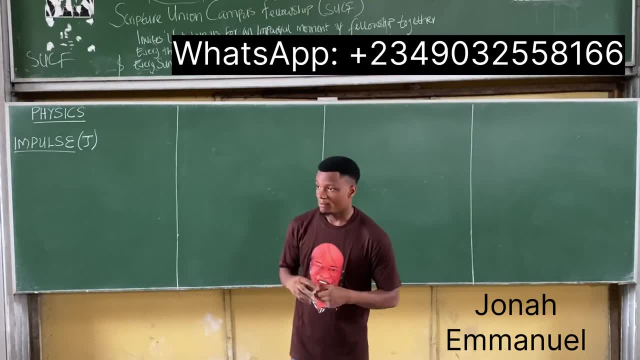 Alright, so impulse is represented using J, not the usual I. alright, I know most people use I for impulse, but I is usually for moment of inertia. but whichever way, we could still use I if you want to. alright, So irrespective of your representation, we can use generally impulse. 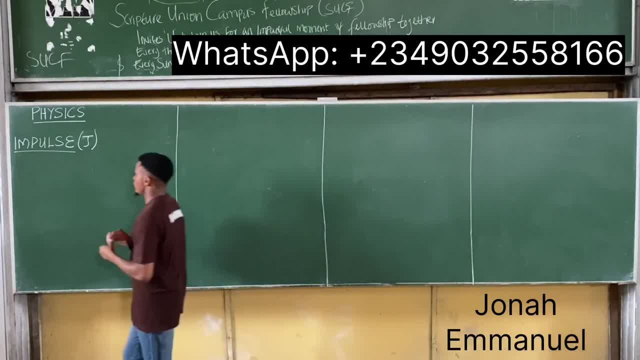 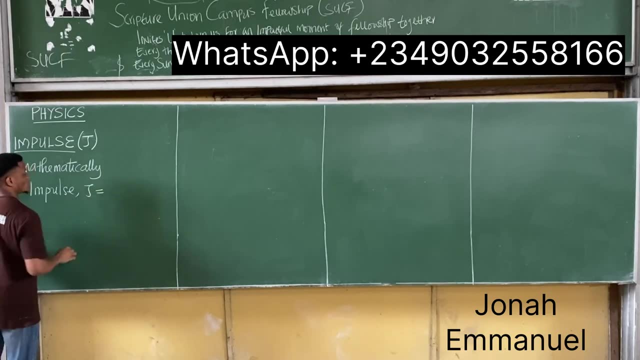 is usually J. Okay, so, having said that, we are saying that mathematically, mathematically, impulse, that J is equal to the product of the average force acting on a body or a particle and the time interval with which the force acts. So, impulse is equal to product of force and time. 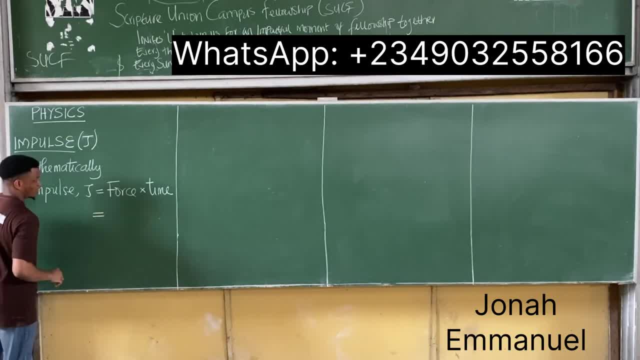 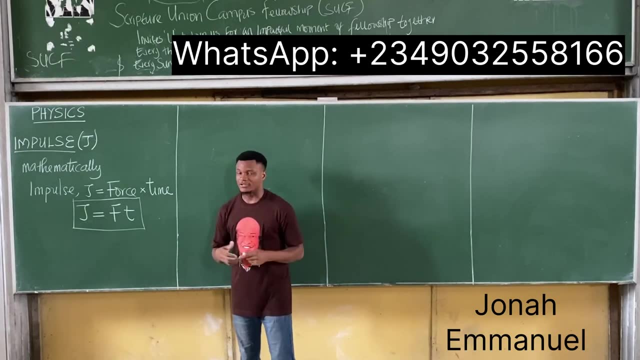 So if this is true, that means that impulse my SI unit becomes. okay, let's say J is equal to Fc. alright, This becomes the mathematical expression for impulse force times time, Because force in Newton, time in seconds. basically, Now, if this is true, let's get the SI unit for impulse. 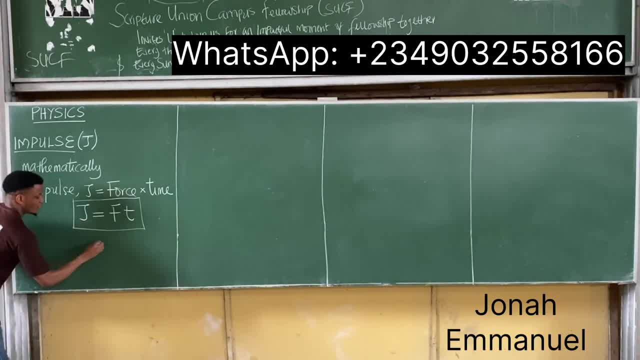 When it comes to impulse, my SI unit becomes: we said force, force is measured in Newton and then time in seconds. So if I say force times time, it means Newton for force times, seconds for time. So hence we're saying that the SI unit, the SI unit of J impulse is Newton seconds, Newton seconds. 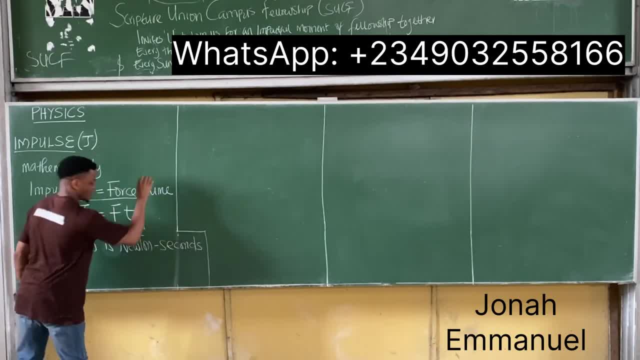 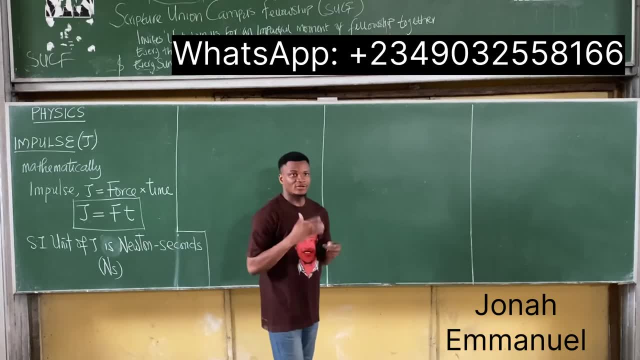 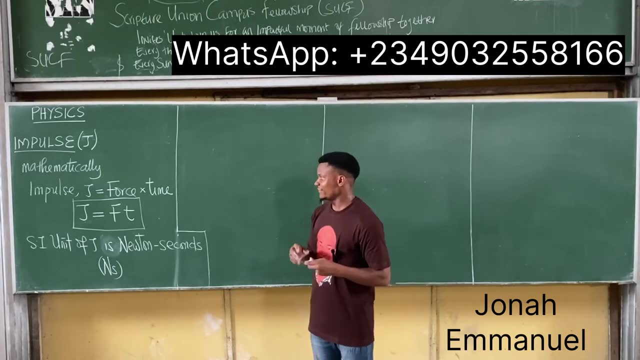 Newton seconds. that's NS as your abbreviation. Alright, so that's this. Now there is something about impulse and momentum. alright, Impulse and momentum are related. related in the sense that they have the same SI unit, technically, and also the same dimension. 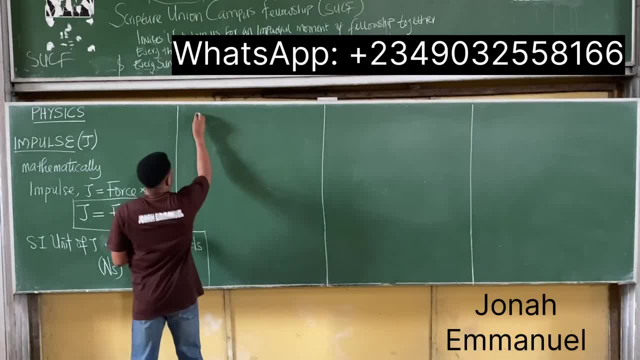 okay, Let me show you how that works. So we said: momentum P is equal to. we said: momentum P is equal to the product of mass and velocity. and we said: for mass, your SI unit is kilogram, velocity is meter per second. So we got the SI unit of impulse as of momentum, as kilogram meter. 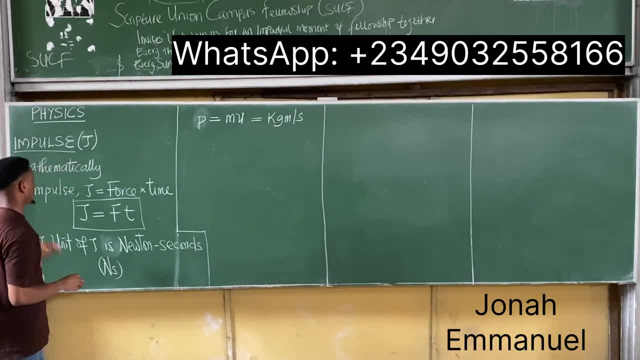 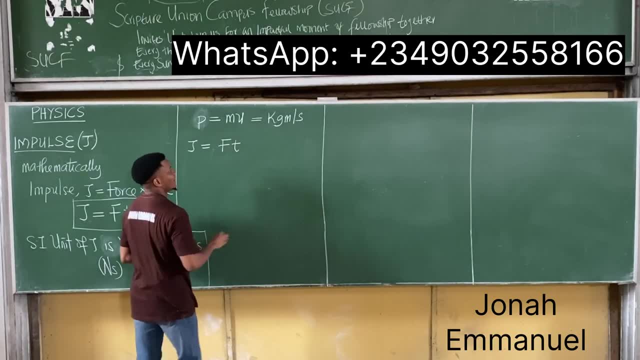 per second. Let's look at the SI unit for impulse. For impulse J we said it's equal to the product of force and time. and that's equal to force was in seconds, force was in Newton and time in seconds. The question will now be: how are these two having the same SI unit? 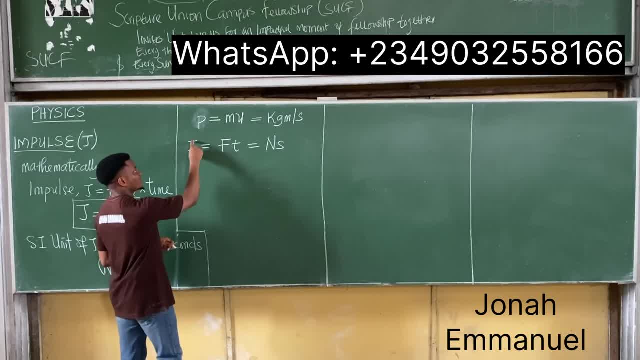 Well, let's look at this. Let's break this down a bit. Let me show you how impulse and momentum have technically the same SI unit. Now let's break this down. First things first. what's force? We said force. from Newton's law of motion we know that force is equal to the product of mass. 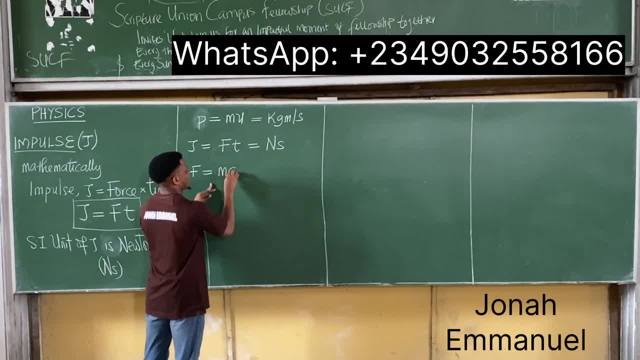 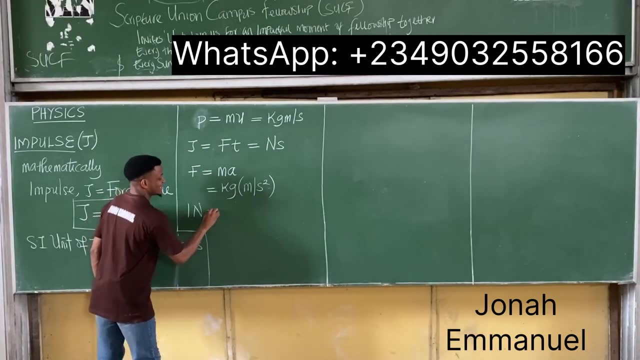 times acceleration. So force is equal to mass times acceleration. Now, if this is true, mass is measured in kilogram, while acceleration is measured in meter per second squared. So we're saying that one Newton is the same thing as saying one kilogram expanding this one kilogram than this. 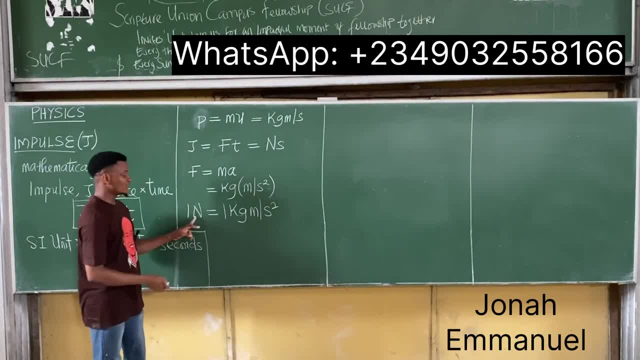 meter per second squared. So Newton and kilogram meter per second squared are the same thing. In other words, if I say that momentum, if I say that impulse J is equal to force, times time that can still be written as being equal to force- is kilogram meter per second squared. 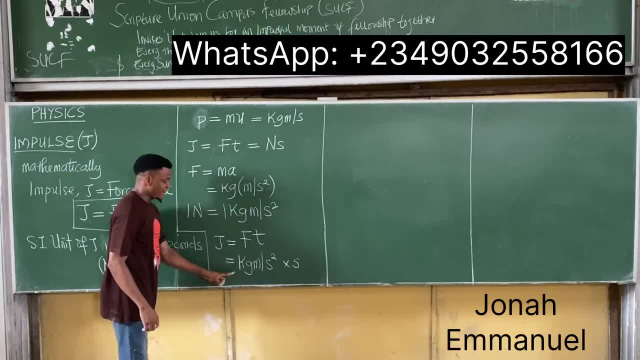 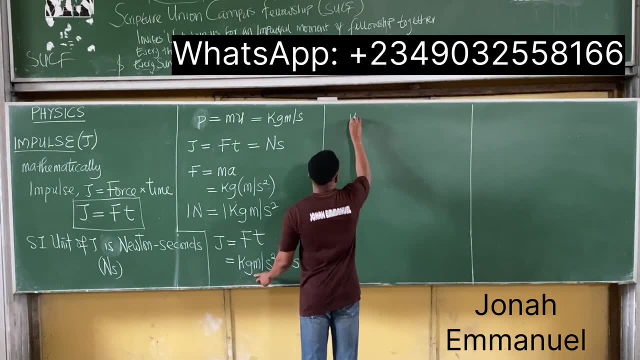 times time in seconds. If I rewrite this one here in terms of a fraction having numerator and denominator, that means impulse becomes kilogram meter all over second squared. That's what I have here multiplied by second. From here, second here, one second here. 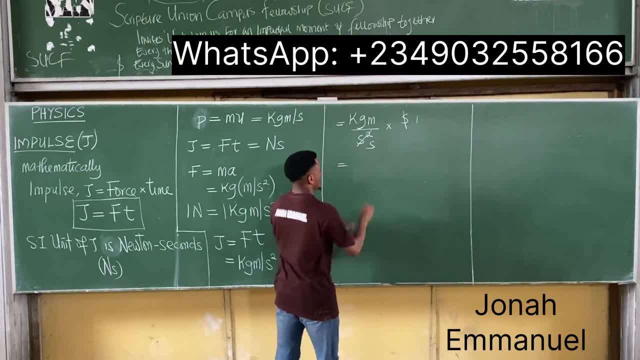 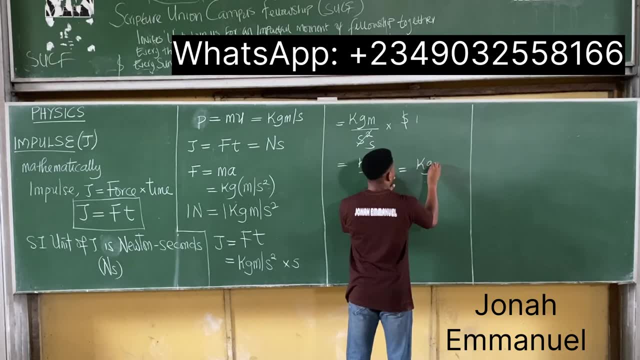 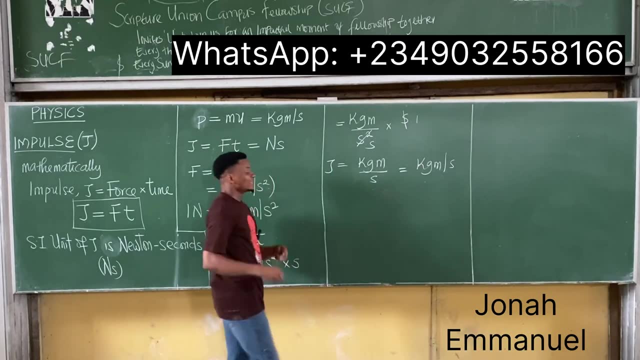 here s. So this can cancel one of this. That becomes kilogram meter per second and that's equal to kilogram meter per second. So you can see that from here that momentum and impulse have the same SI unit. So we can say that momentum and impulse, since they have the 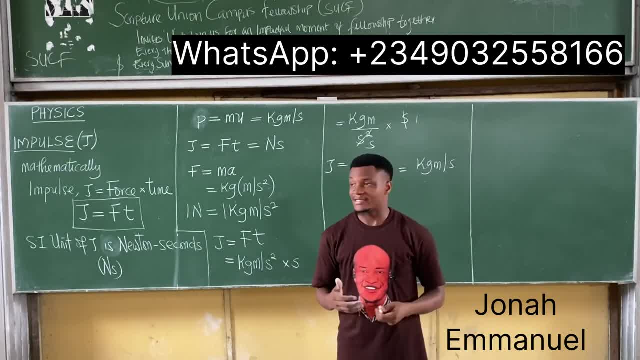 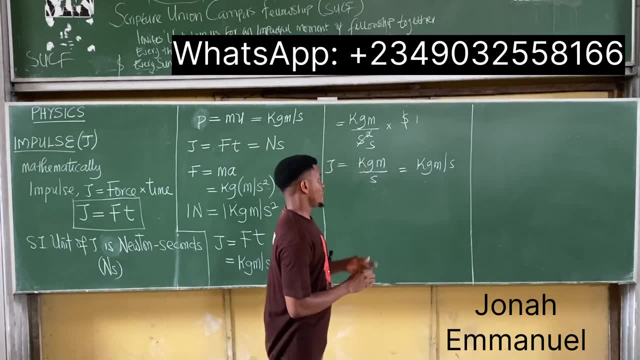 same SI unit, they will have the same dimension. So we can say: impulse and momentum are dimensionally homogeneous. Now the question is this: If impulse and momentum have the same SI unit, are there any difference? Is there a difference between impulse and momentum, Or are they exactly? 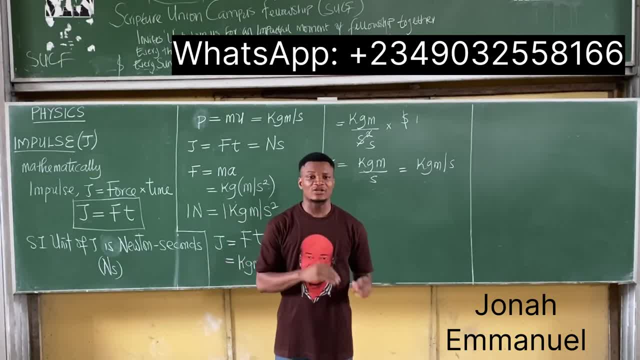 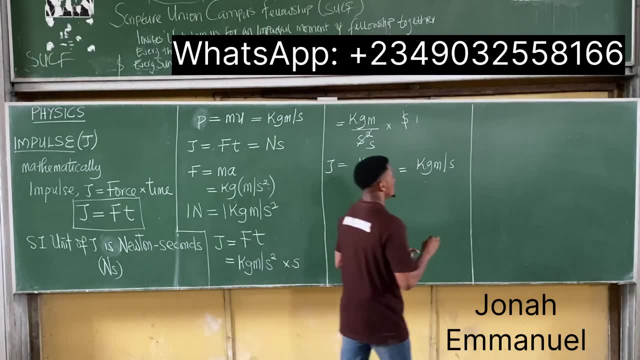 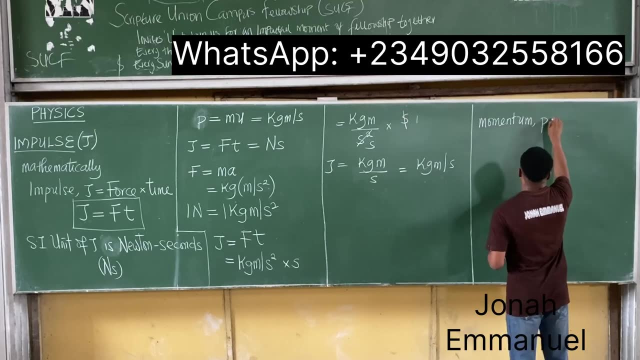 the same thing? Now, the answer to that question is this: Impulse and momentum are not exactly the same thing. All right, Here's what to note: Momentum: here's what to note. Momentum, that's p, is equal to the point. So p is equal to the point of the momentum and momentum is equal to the point. 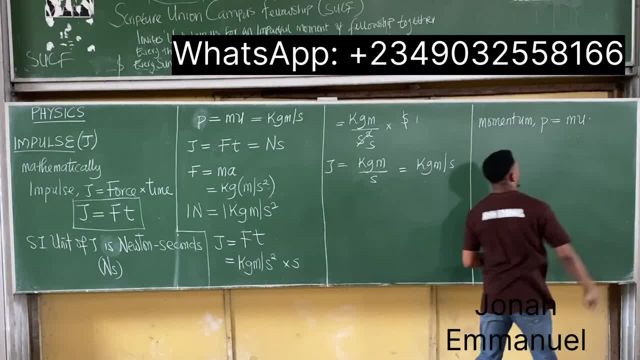 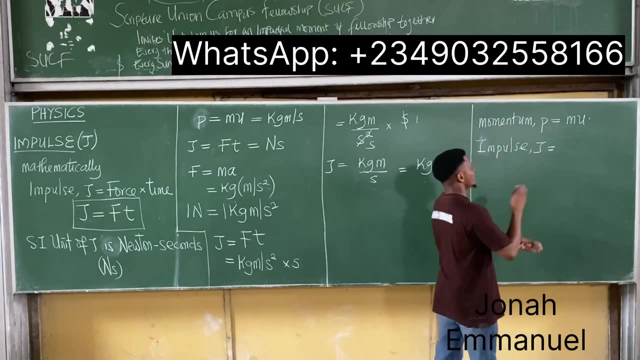 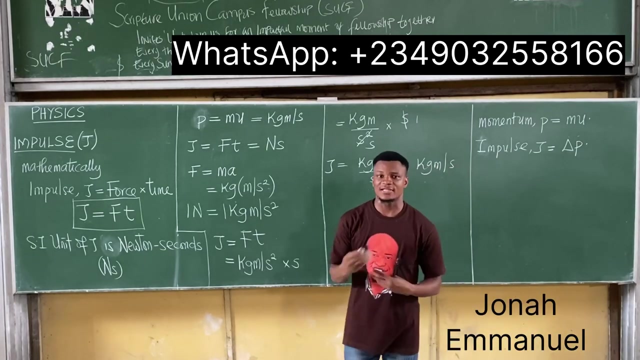 product of the mass and the velocity of a body. why impulse? okay, why impulse that j is equal to force, times, time. or, if I want to relate this to momentum, impulse is simply a change in momentum. Please note this: Impulse is simply a change in momentum. So I'm saying: 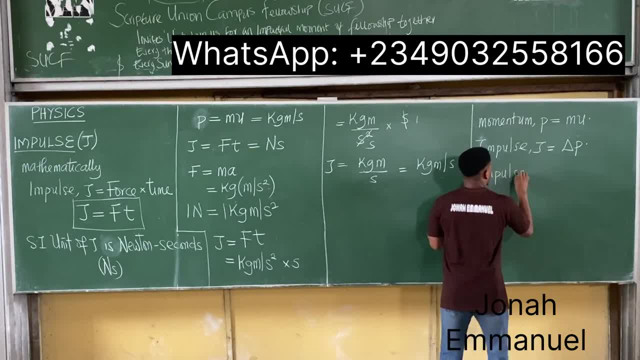 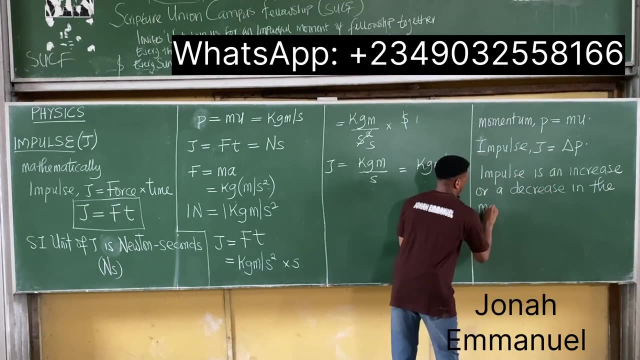 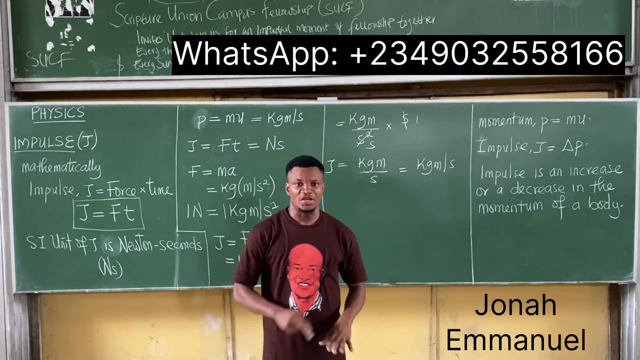 this: that impulse is an increase or a decrease in the momentum of the body. Alright, so please note this: that impulse is simply an increase. So this is what differentiates impulse from momentum. Yes, there's a similarity, which is that they have the same SI in it, as I've showed you here, and also they will have the 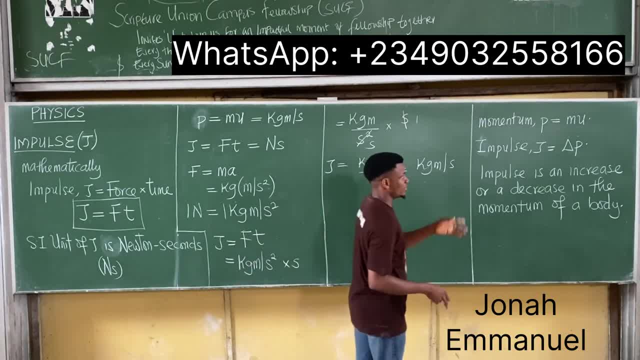 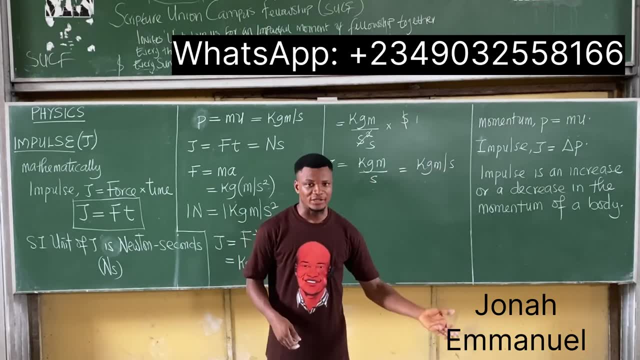 same dimension. But then the little difference between impulse and momentum is that, while momentum is just simply the product of the mass of a moving body and its velocity, impulse is really a change in the momentum. all right, So impulse is an increase or a decrease. Therefore, impulse is a change in momentum. 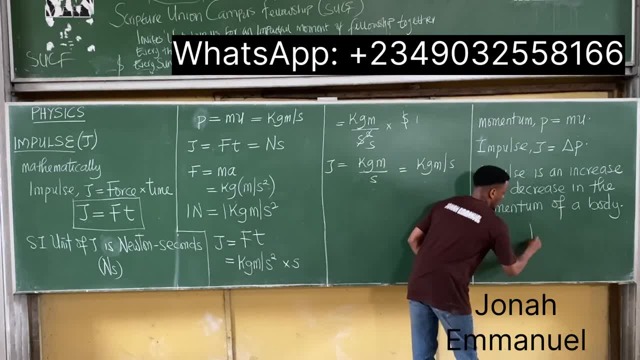 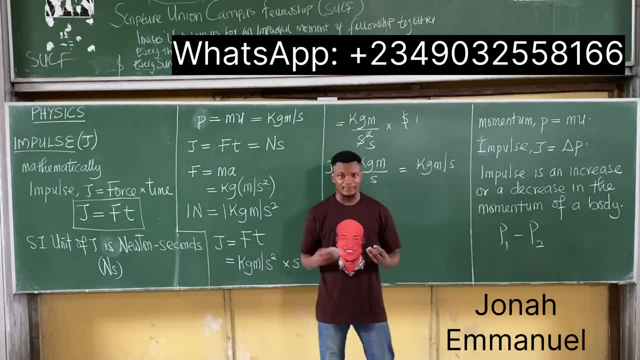 Now, let's say a body has a particular momentum- let's call it P1, initial momentum, P1, and then later has a second momentum, let's say P2.. This one- here- the difference between P1 and P2, represents the impulse of the body. all right, So impulse is simply a change in. 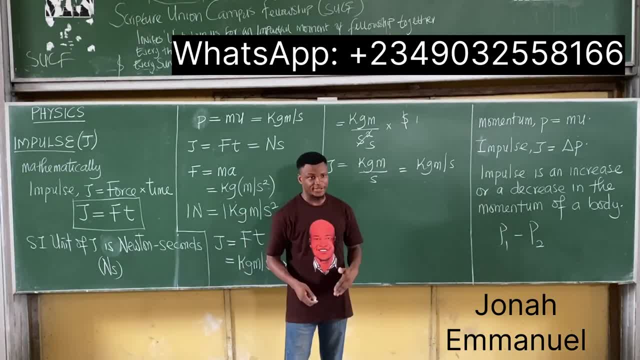 momentum, whether it's an increase or a decrease. So far as it's a change in the momentum of the body, we say impulse has occurred. Now, if this is true, let's say there's an change in momentum. For example, let's say: 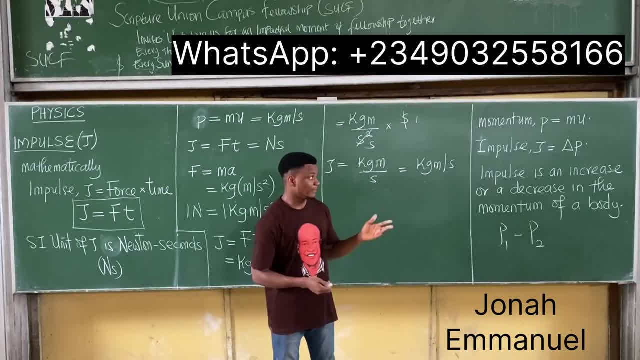 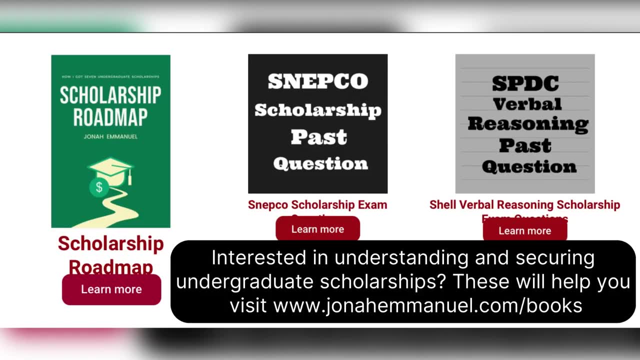 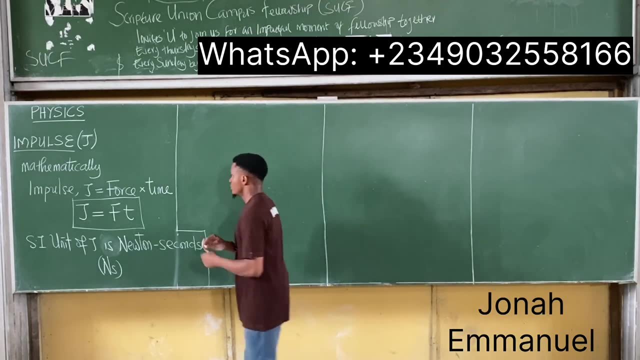 you're in the middle of a stage Now. you're running in the middle of a stage. you're running. let's take just some few problems on impulse and see how we can solve problems involving impulse. Okay, let's take a first example on impulse. Let's say a force of 200. 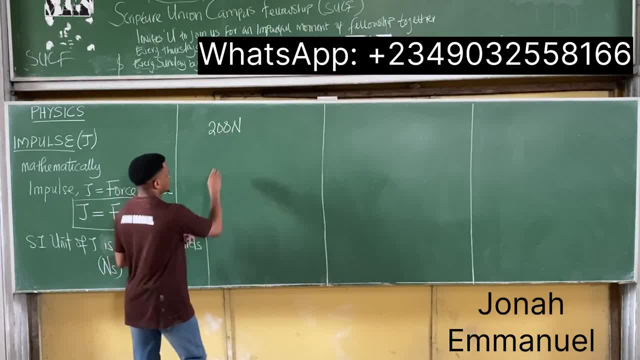 Newton acts for, let's say, 3.5 seconds. What will be the impulse? A force of 200 Newton acts for about 3.5 seconds. What will be the impulse For this? we say the force is already 200 Newton and the time is equal to 3.5 seconds. The 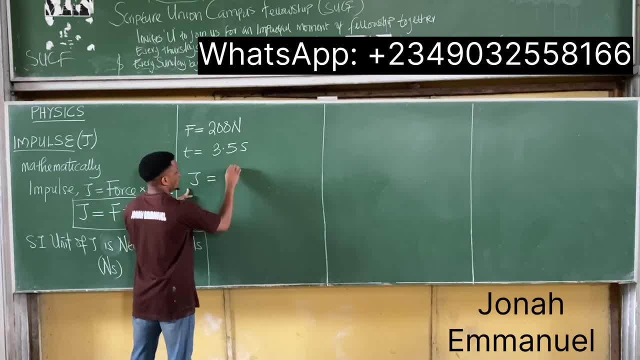 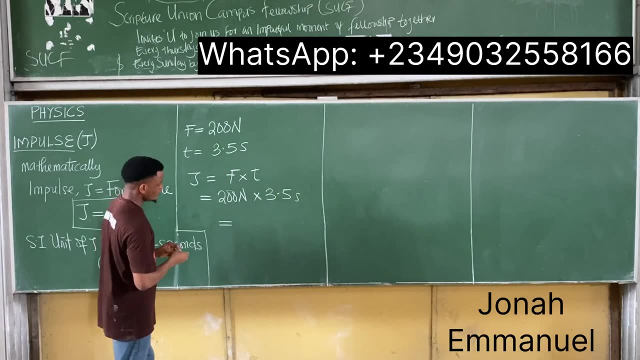 impulse, that's J, is equal to product of force and time. If I multiply this, the force is about 200 Newton. multiplied by the time it's about 3.5 seconds. So multiply this, I have 700 Newton seconds. So we can say that the impulse is equal to 700 Newton. 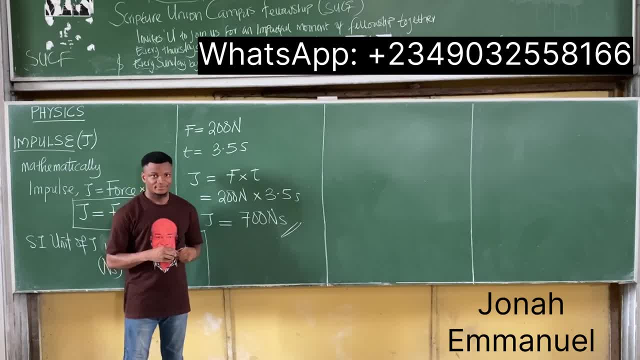 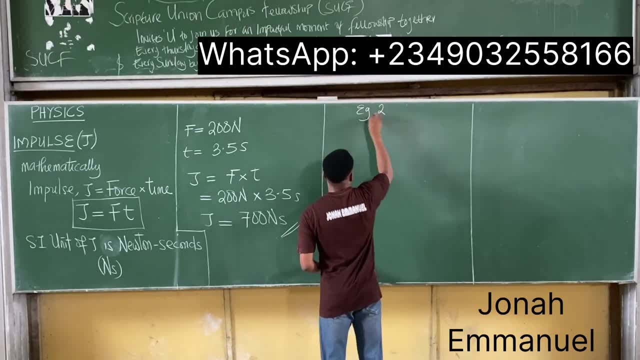 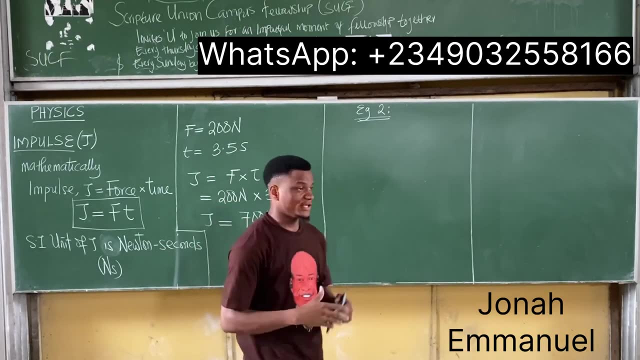 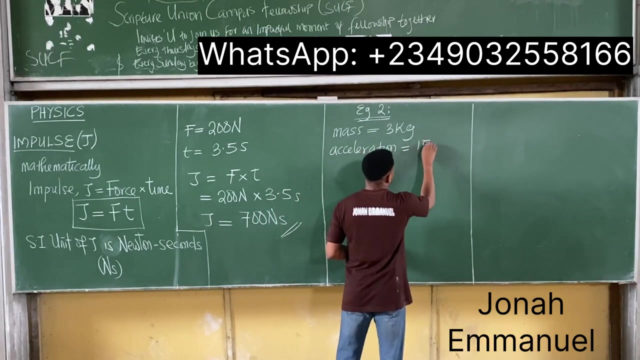 seconds as my answer. Okay, so let's take a second example Now. in this example, let's say we have a force. Okay so example two: If a mass of, let's say, 3 kilogram accelerates for, let's say, 15, or accelerates at 15 meter per second square for a time interval of, let's say, half a century, 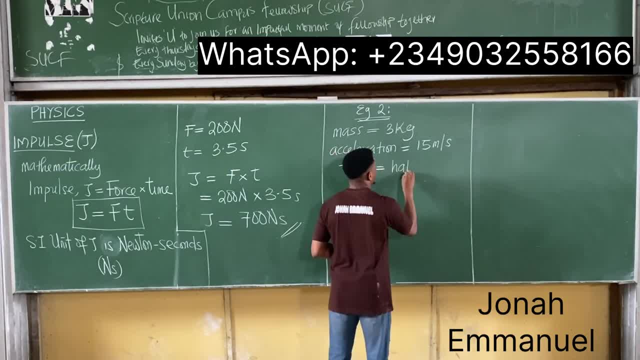 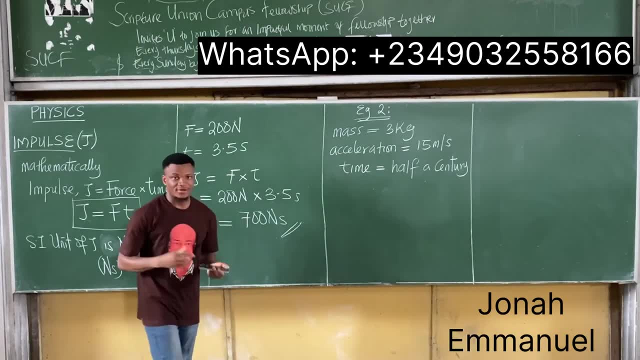 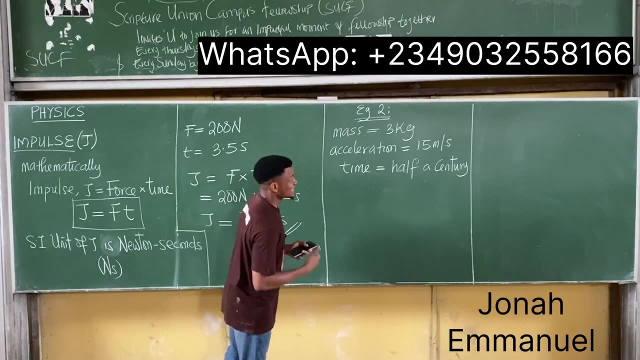 for a time interval of, let's say, half a century. What's going to be the impulse created, All right. so a mass of 3 kilogram accelerates for like 15, or accelerates at 15 meter per second for half a century. What will be the impulse? So for this, 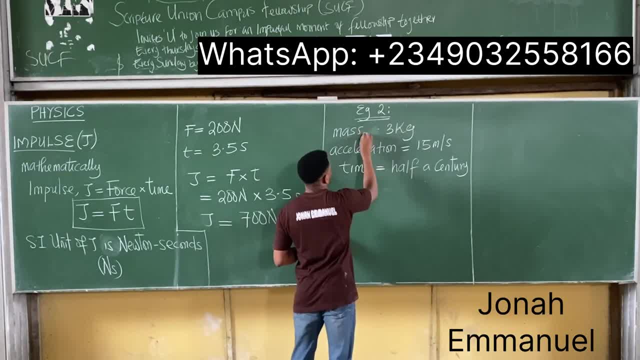 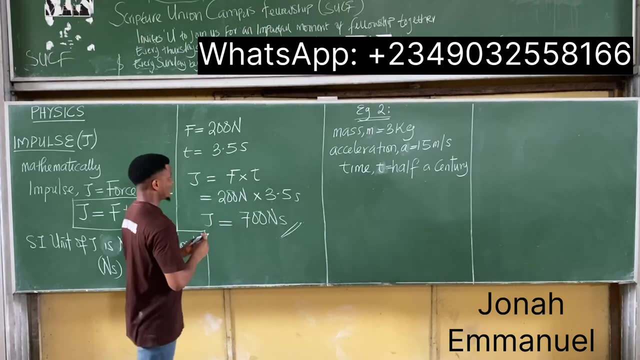 question: how do we solve this? First is first The mass- let's call these M acceleration, And the time interval- let's call this c. okay, It's got to have a century, All right, So we have this. 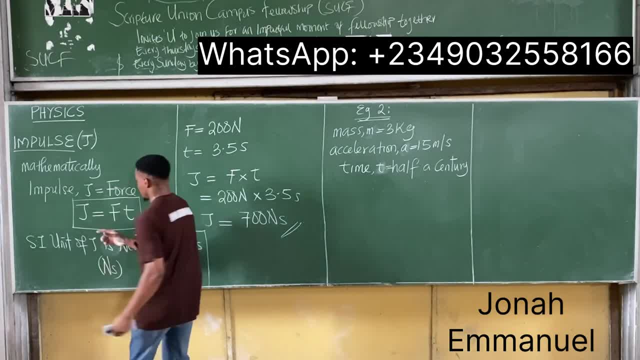 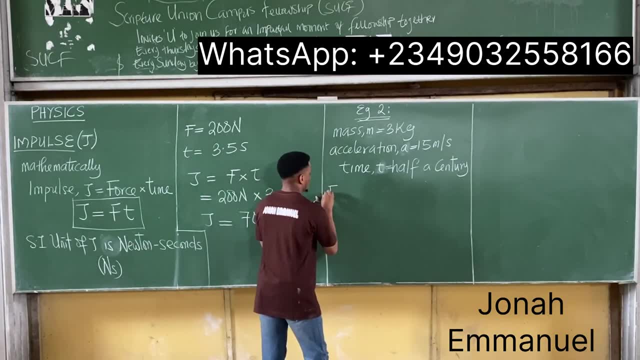 First things first. we know that impulse is equal to the product of force and time. So first things first, let's get force. The force will be equal to mass times acceleration from Newton's second law of motion, And that's equal to mass. 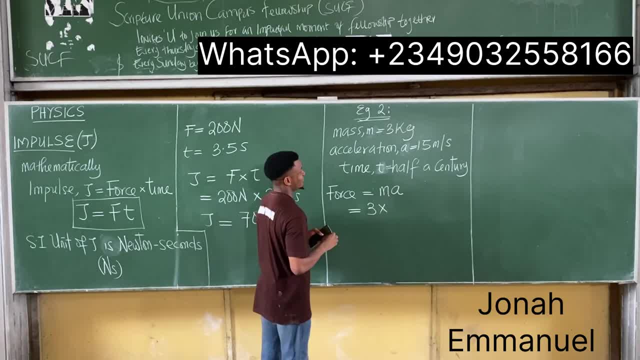 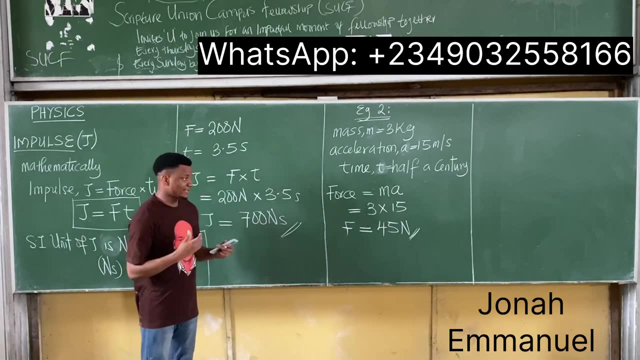 The mass is 3 kilogram times acceleration. Acceleration is about 15,. okay, So if I multiply this, it means that the force is equal to 45 Newton. All right, 45 Newton becomes the force That's 3 times 15.. 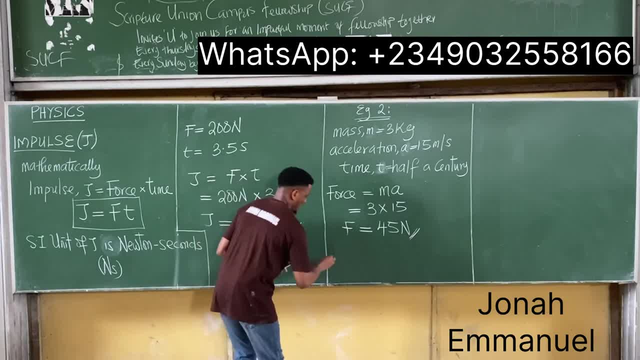 I have 45.. Next up, let's get the time. The time is equal to have a century. So the question now is this: How, How many seconds do we have in half a century? How do we calculate that? Now, that's quite simple. 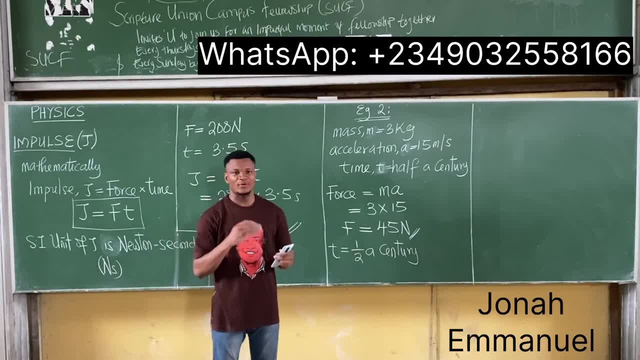 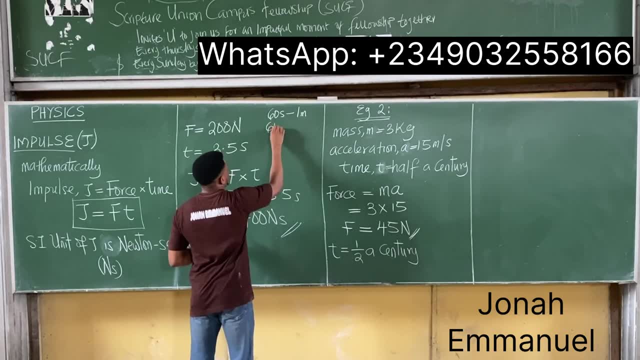 To get the number of seconds in a century, we use a very popular rhyme And the rhyme is this: that 60 seconds make 1 minute, 60 minutes make 1 hour. So the 4 hours make 1 day, 7 days make 1 hour. 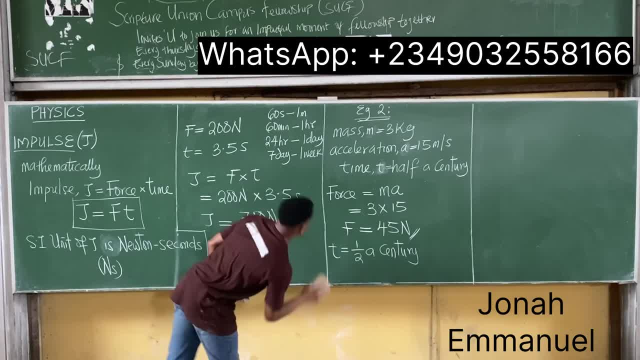 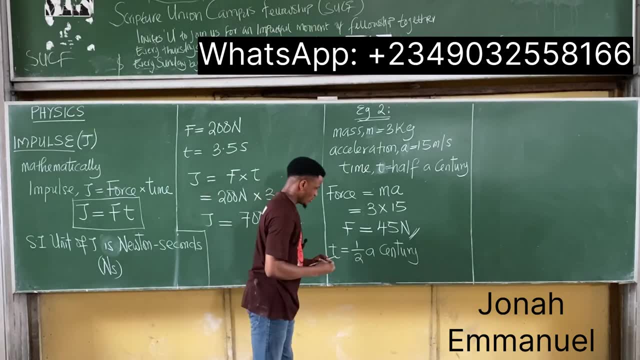 So we have this All right. So first is first: When we say half a century, what do we mean? Half a century is simply equal to a century is 100 years. All right, 100 years make a century. So when we say half a century, that's equal to half times 1 century is 100. 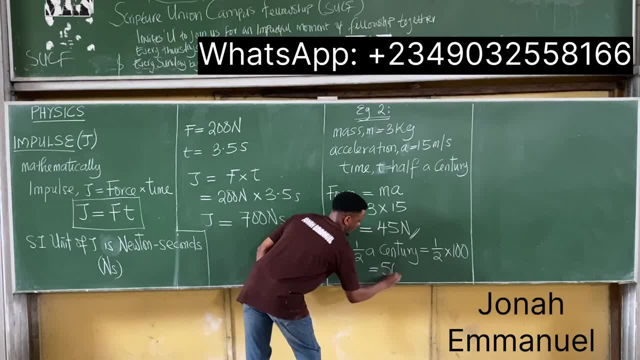 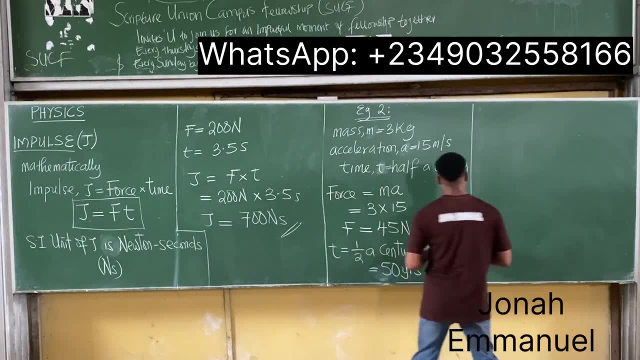 In years. half of 100 gives you 50 years. All right, So half a century is 50 years. Now, if this is true, how do you calculate the number of seconds in 50 years? We use a popular rhyme. 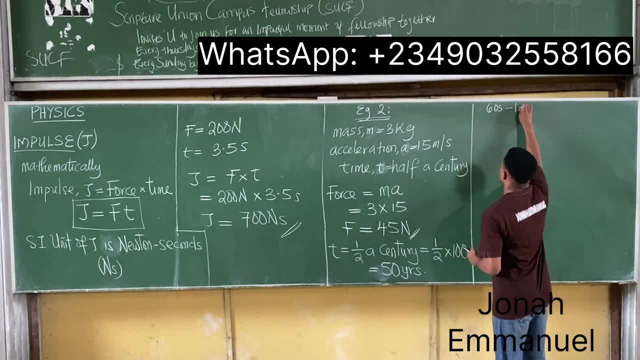 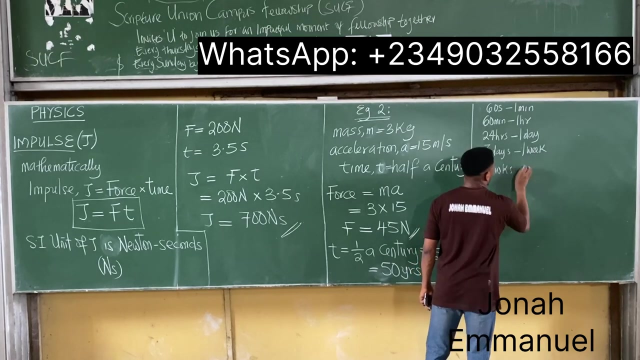 And the rhyme is this: that 60 seconds make 1 minute, 60 minutes make 1 hour, 24 hours make 1 day. So that's 50 years. 7 days make 1 week, 4 weeks or better. instead of using 4 weeks, we can just use 52 weeks makes 52 weeks. 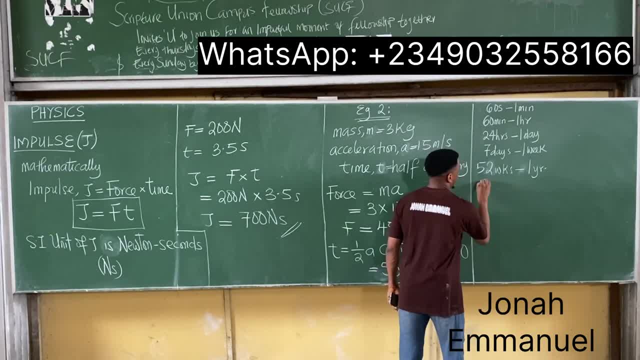 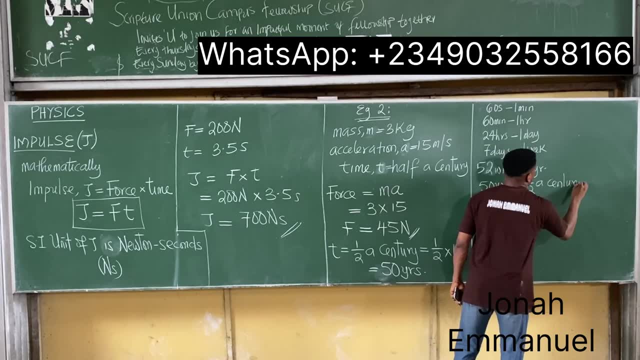 make 1 year And, of course, 50 years make half a century. All right, So that's: 50 years Make half a century, All right, So 50 years make half a century, All right, So we have this. 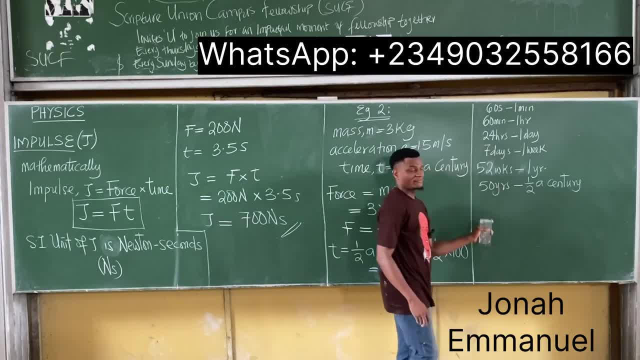 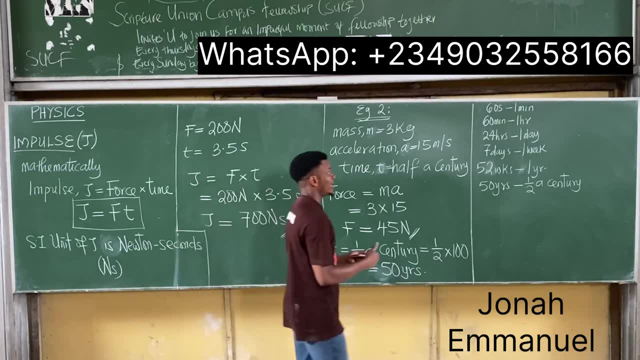 That means if you have to come to half a century. so this is like an idea of how to do conversion in time. All right, So use this rhyme and see how you can fix that up as part of the rhyme. So I have 60 seconds. make 1 minute. 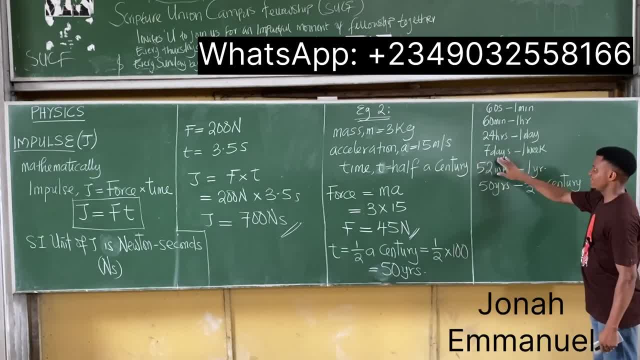 60 minutes make 1 hour. 24 hours make 1 day. 7 days make 1 week, 52 weeks make 1 year. So I assume they are said: a century Out of 15,. 100 years make 1 century. 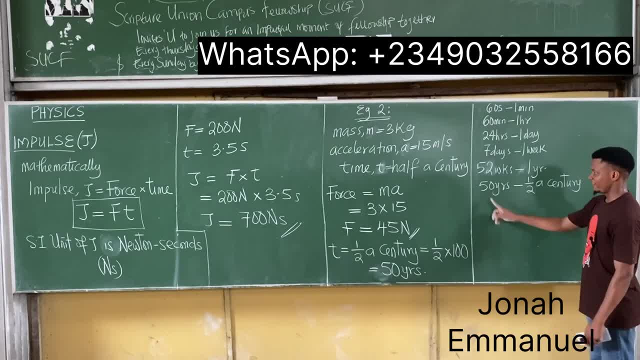 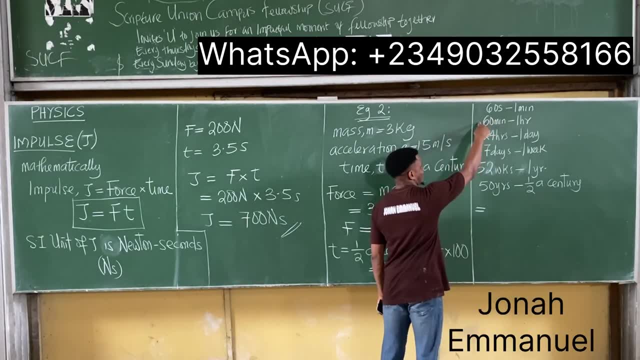 But they ask for half a century, So I'm using 50 years make half a century, So to get the number of seconds in half a century becomes this times, this times, this time, this time, this time, this, And that becomes 60 multiplied by this one here. 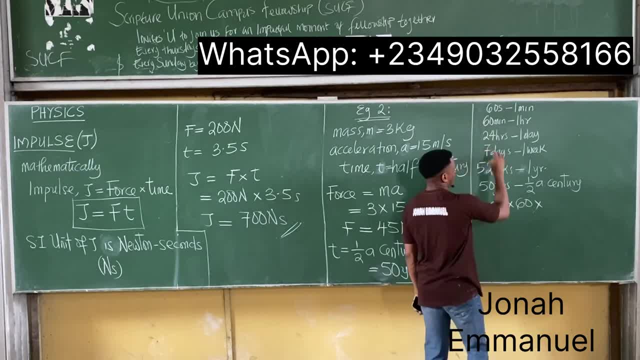 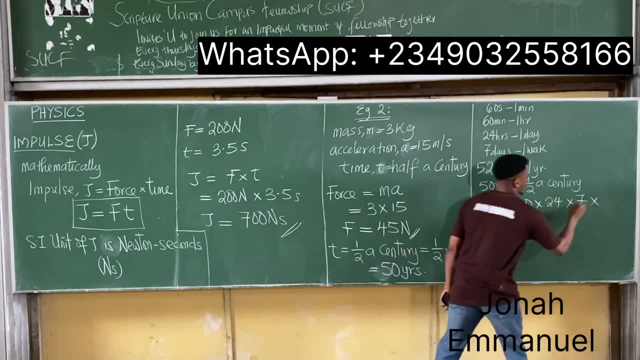 60.. Multiplied by this one here: 24.. Multiplied by this one here: Seven. Multiplied by this one here: 52.. Multiplied by this one here, multiplied by this one here: 50. and that's equal to so if i multiply all of this. 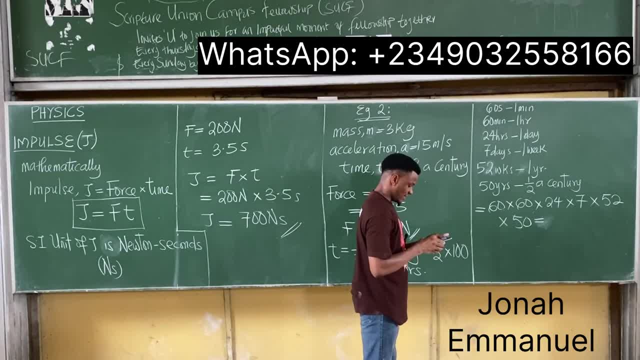 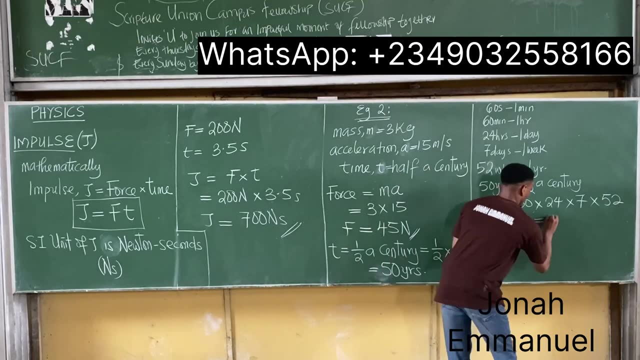 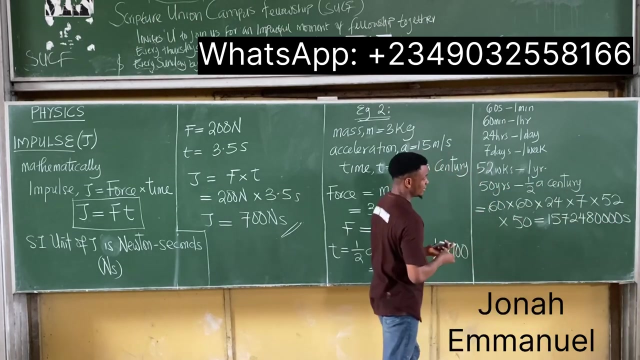 what do i get? so i'll use my calculator. so i'm having 60 times 60 times 24 times, 7 times 52 times 50, that gives me about 1572. four eight zero, zero, zero, zero, second. so this is the time in half a century. one. let me just 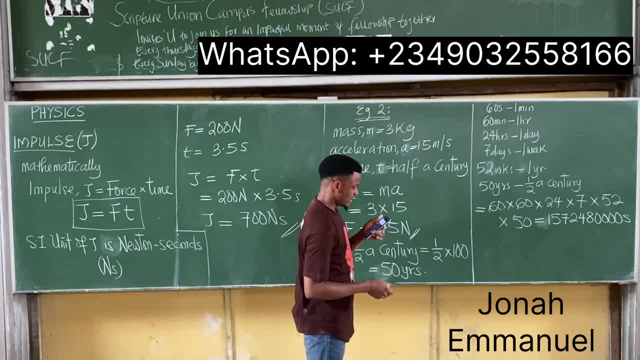 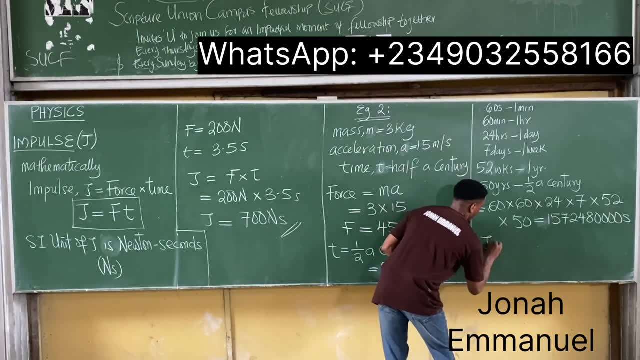 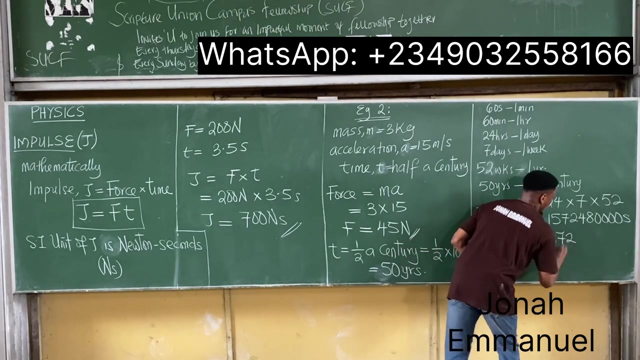 confirm that one, five, seven, two, four, eight, zero, zero, zero, zero. okay, so we have this as a time, so hence we'll have that. the impulse j is equal to force. the force again is um 45, so it becomes 45 multiplied by the time interval in half a century. one, five, seven, two, four, eight, zero, zero, zero, zero. and if i multiply this it: 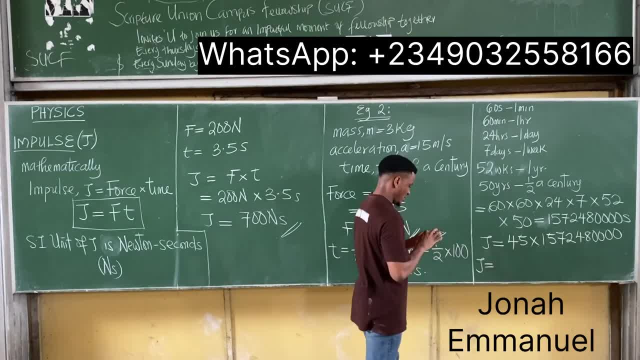 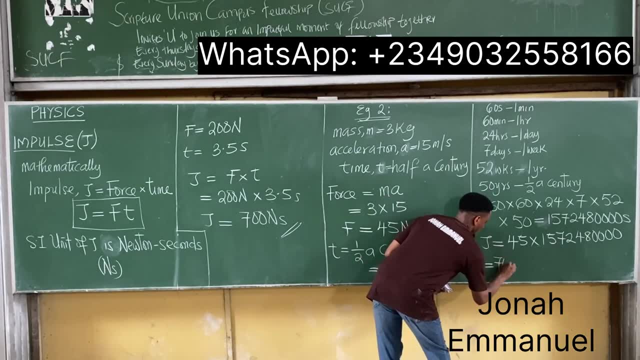 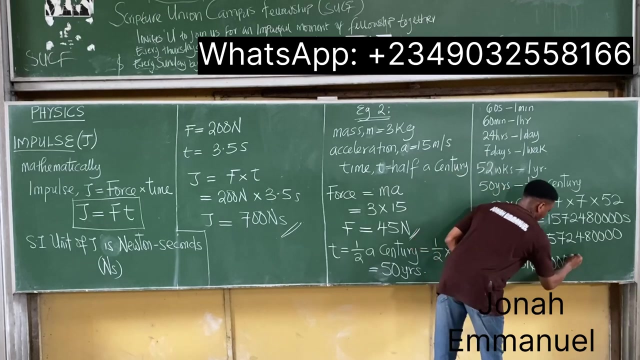 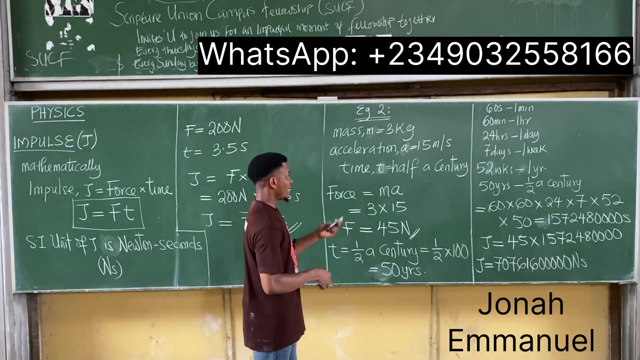 means that impulse j is equal to um two times forty five. i have about seven to seventy six, seventy seventy six, one, six, one, six, um one, two, three, one, two, three, four, five. this man is in newton seconds. so this is the value of the impulse. after half a century now, this value is too big. let's convert it, let's. 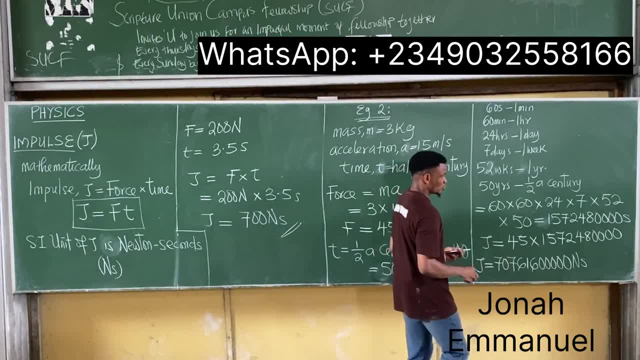 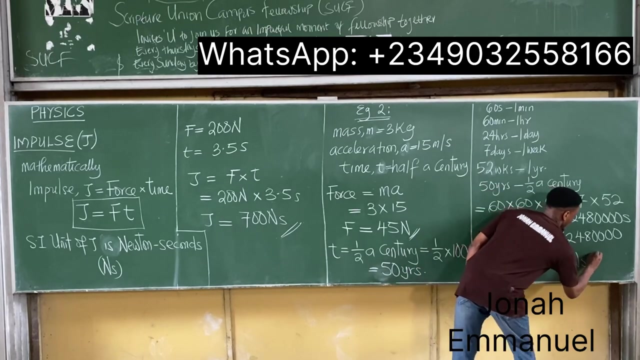 convert it: um, let's give the prefix. so to give this a prefix, this becomes from here: if i move: one, two, three, that's kilo. one, two, three, that's uh, mega, that's six, now mega. one, two, three, that's nine, now that becomes giga, it becomes seventy point. seventy six approximately, that's equal to seventy point. 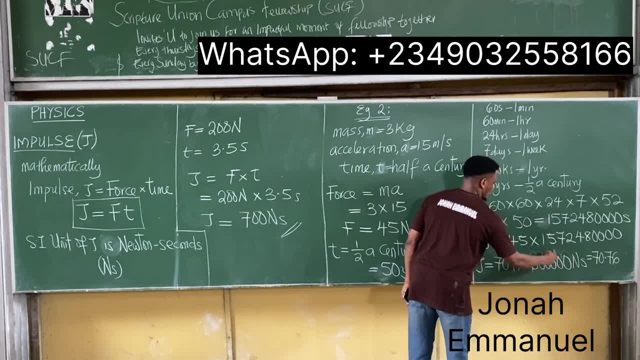 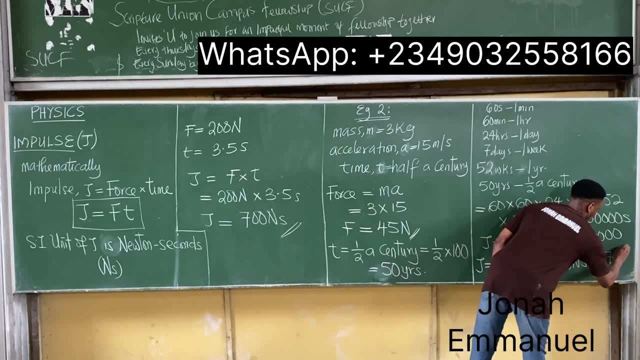 seventy six. so i move nine times: one, two, three, four, five, five, six, seven, eight, nine, seventy point seven, six. that becomes giga. it becomes a giga newton. okay, beta, still let me write it down for clarity: that would be equal to 70.76 giga newton seconds. all right, so this becomes the value of the impulse. so, as an scrub, notice that you can notice thatORD we have a pattern: one plus two plus three plus four plus five plus five plus eight plus eight plus seven will be 7.688 미 bonds. so that our impulse value That's 70.76000. manga in and minusrum- who is neverbuyguide- of 70.76000, indeclaired of 70.776. 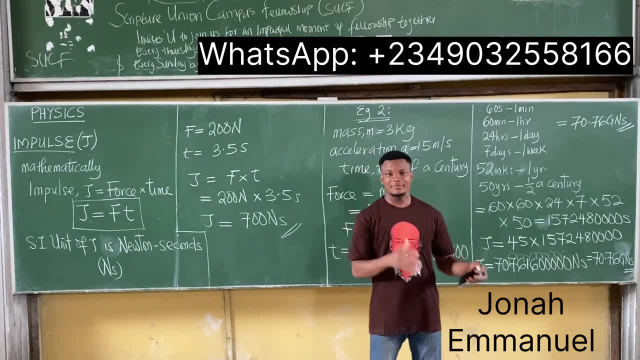 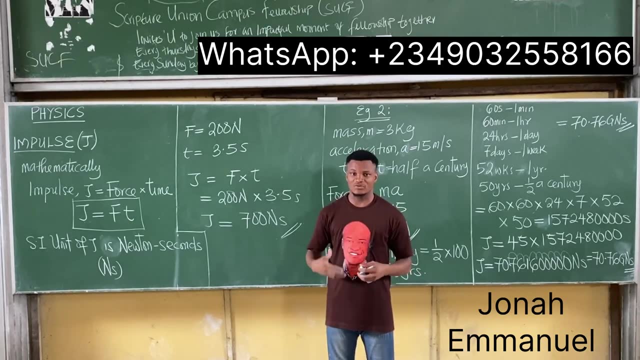 So I've covered major topics on physics and chemistry, including mathematics, for O-level students, alright. So if you want to check out all my videos, I have about almost 50 videos, 50 plus videos for O-level students when it comes to physics or on physics, chemistry, mathematics and the likes. 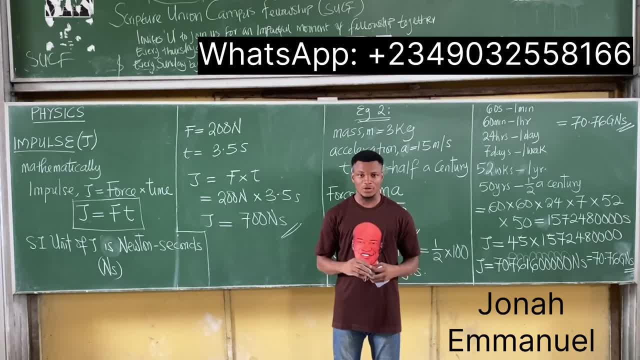 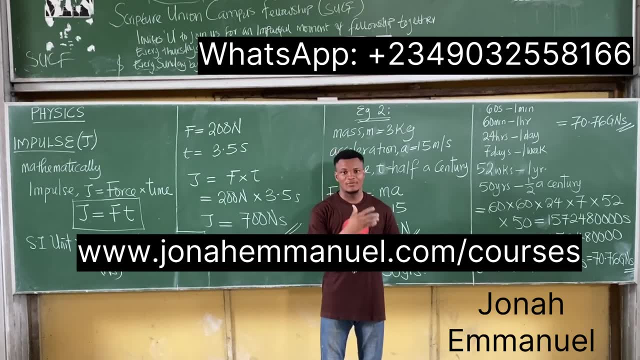 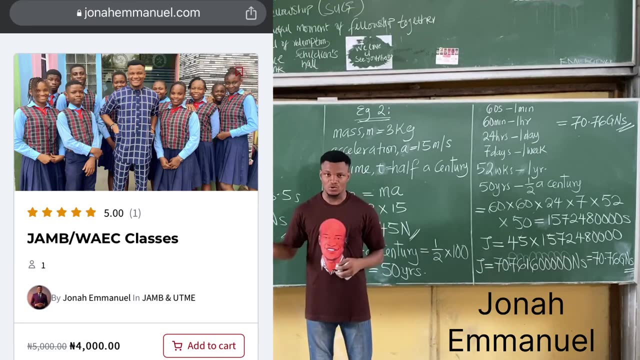 If you want to access my full 50 plus videos on physics, maths, chemistry, simply visit my website, wwwjunainmanuelcom. forward slash courses and pick the jam slash wire classes and to give you access to all my classes. alright, 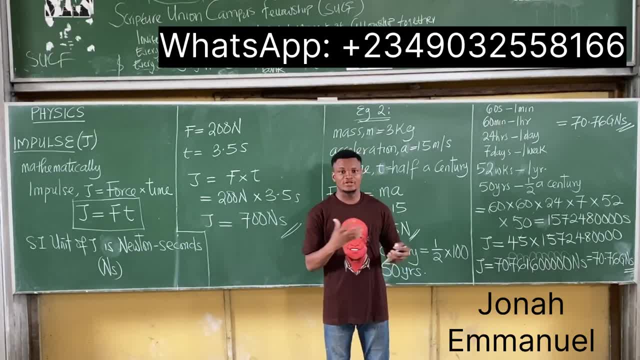 Alright then. so in the next class we'll look at the concept of Newton's laws of motion. See you in the next class.